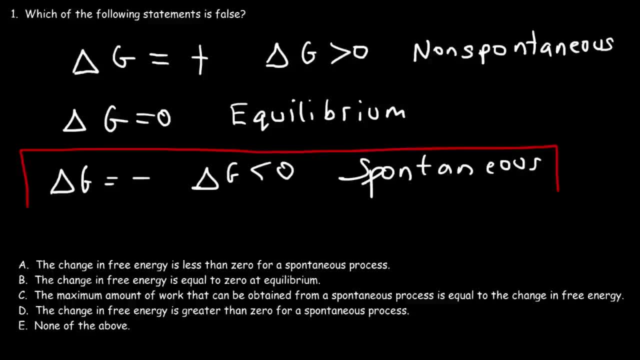 it's usually associated with a spontaneous process, So that's something you want to keep in mind. So which answers are true and which ones are false? So let's look at A. The change in free energy is less than zero for a spontaneous process. 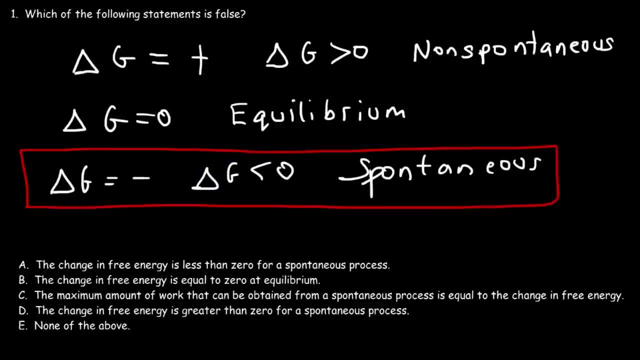 That's true. Looking at B: the change in free energy is equal to zero at equilibrium. That's also true. So we're looking for the false statement. And C: the maximum amount of work that can be obtained from a spontaneous process is equal to the change in free energy. 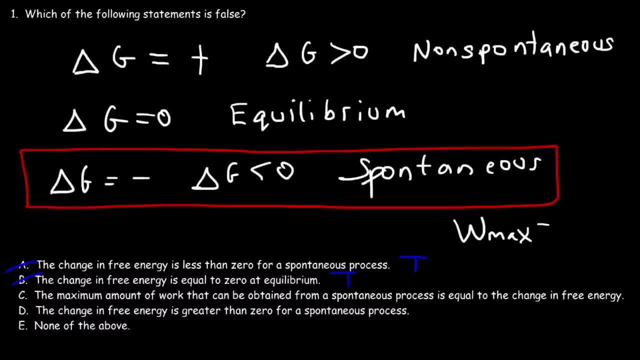 That is also true. The maximum work that can be obtained is equal to delta G for a spontaneous process. Now, if you have a non-spontaneous process, to make it work you got to put energy into it, And so the minimum work required to drive a non-spontaneous reaction. 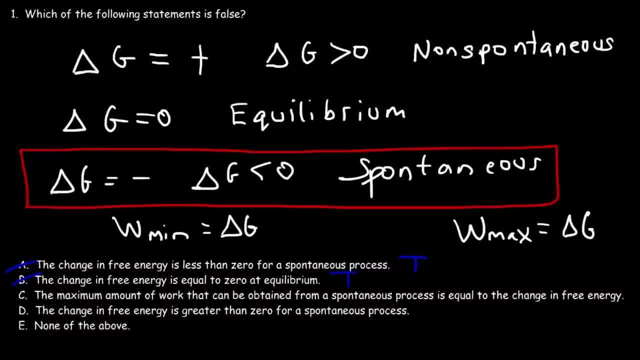 forward is also equal to delta G. Now we use the word minimum because you need to put in energy to overcome the energy losses that occur due to friction. So if you're trying to drive a non-spontaneous process forward, you need more energy than delta G. 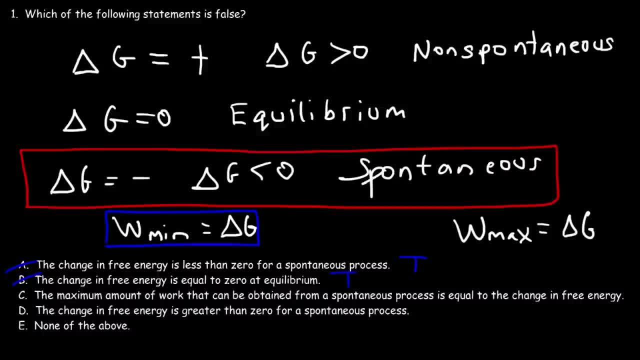 So the minimum amount to get it started is equal to the change in free energy. But if you have a spontaneous reaction where you're trying to get energy from the reaction, then the maximum energy that you can get or the maximum useful work that it can do. 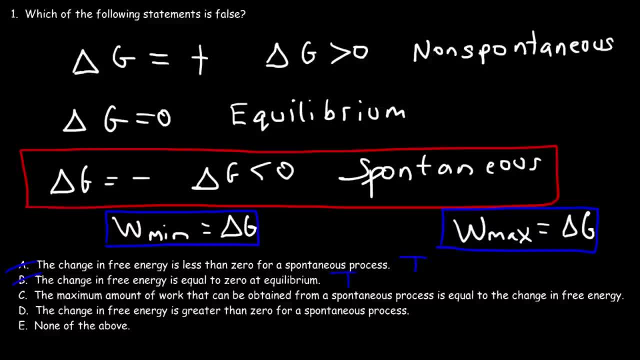 is equal to the change in free energy. So C is a true statement. Now D: the change in free energy is greater than zero for a spontaneous process. It's greater than zero for a non-spontaneous process. so D is the false statement. 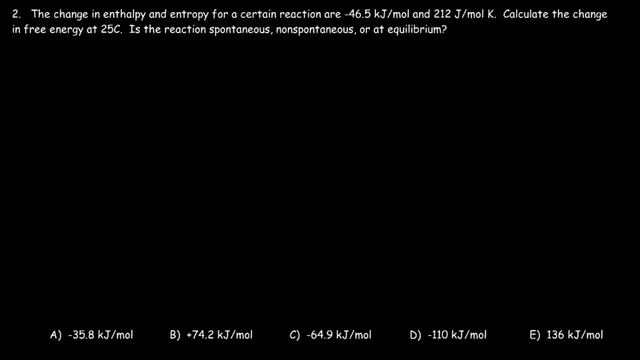 which means D is the answer that we're looking for. Number two: the change in enthalpy and entropy for a certain reaction. are those values Calculate the change in free energy at 25 degrees Celsius? So how can we do this? What formula do we need? 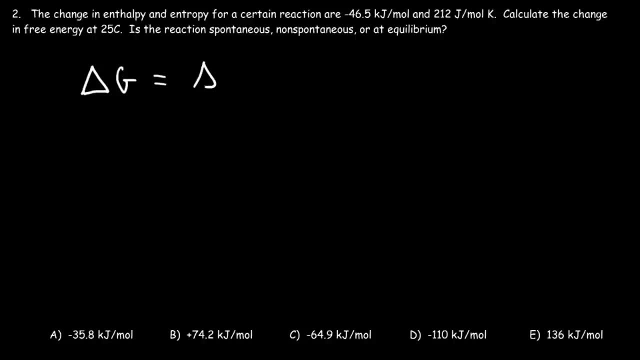 The change in free energy, also known as Gibbs. free energy is equal to the enthalpy change minus the temperature, multiplied by the entropy change. Now you need to be careful with the units. So notice that delta H, the enthalpy change. 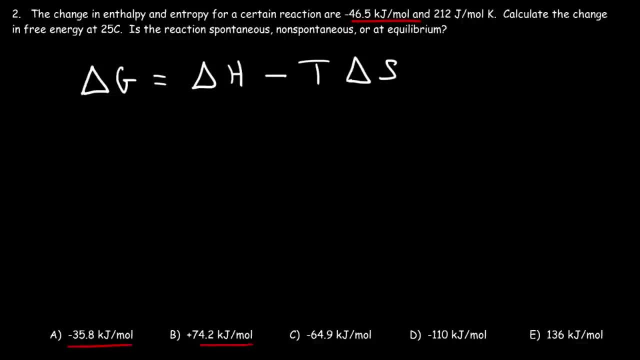 is in kilojoules per mole and delta G is also in kilojoules per mole, But notice that the enthalpy change is also in kilojoules per mole And the entropy change is in joules per mole per Kelvin. 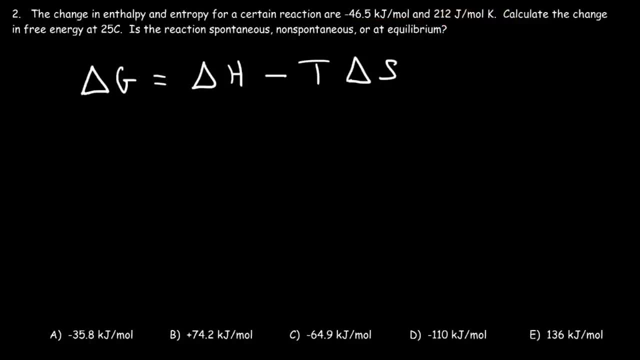 So we need to convert joules to kilojoules And to do that, all we need to do is divide by 1,000.. So let me show you the conversion. So we have 212 joules per mole per Kelvin. 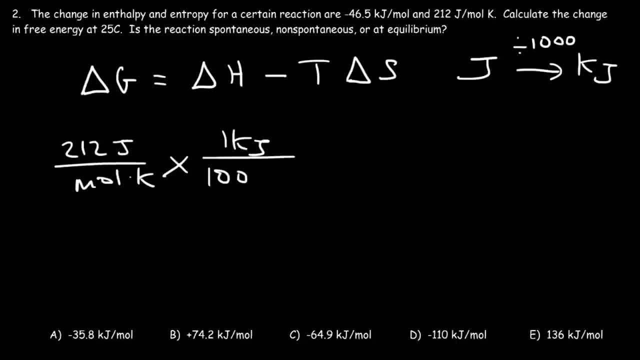 and we know that there's 1,000 joules per 1 kilojoule. So we just got to divide this number by 1,000.. So the entropy change is going to be 0.212 kilojoules per mole per Kelvin. 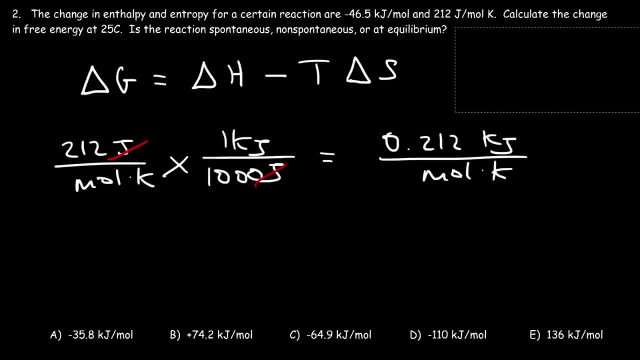 So just keep that in mind. So now let's work on this problem. So delta H is negative 46.5 kilojoules per mole. Now the temperature has to be in Kelvin, So 25 degrees Celsius plus 273,. 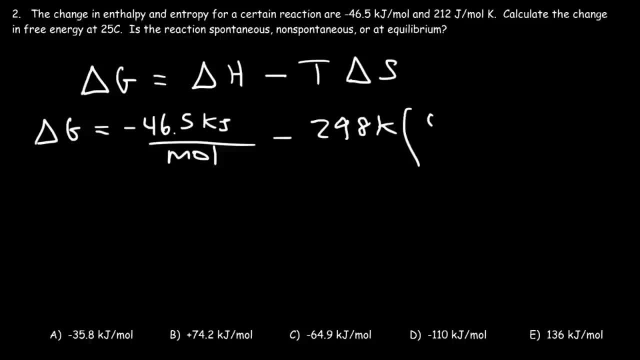 that's 298 Kelvin, And the entropy is 0.212 kilojoules per mole per Kelvin. So notice how the unit Kelvin cancels. And so now this quantity is in kilojoules per mole and this quantity also is in kilojoules per mole. 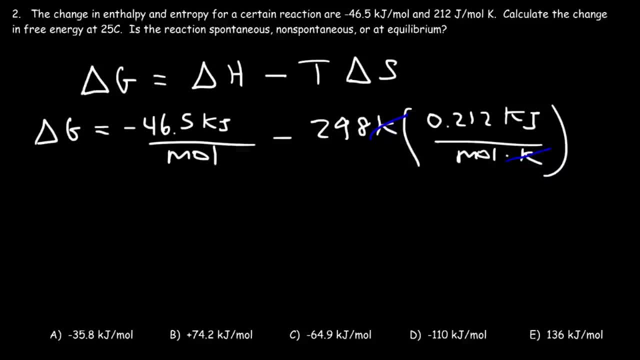 So now let's get the answer. So it's negative 46.5 minus 298, multiplied by positive 0.212.. And so delta G in this example is equal to negative 109.7 kilojoules per mole. 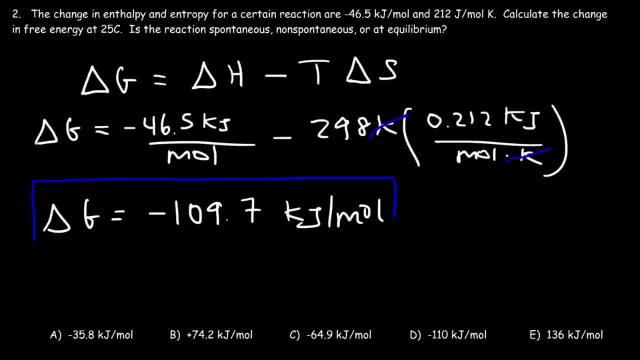 Now, is the reaction spontaneous, non-spontaneous or at equilibrium? What would you say Whenever delta G is negative or when delta G is less than zero? what we have is a spontaneous process, And so that's the answer to the second part. 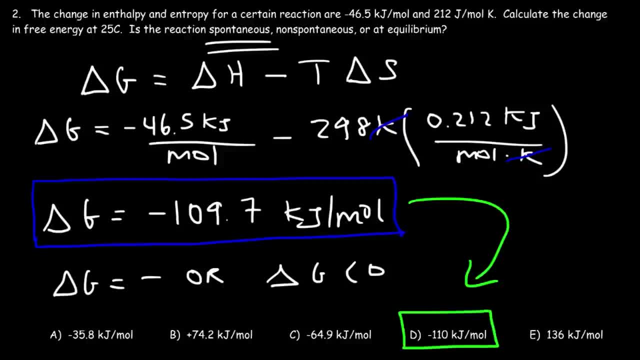 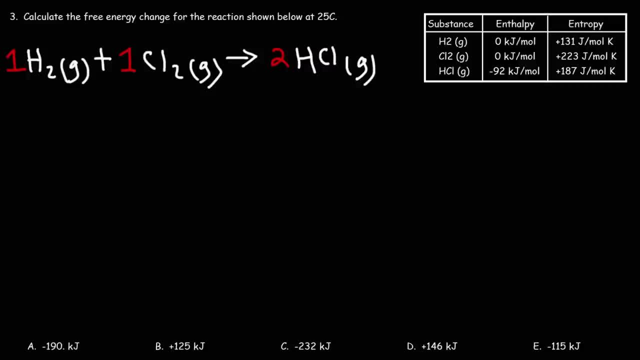 Now this value corresponds to answer choice D, which is rounded to negative 110.. And so that's it for this problem. Number three: calculate the free energy change for the reaction shown below at 25 degrees Celsius. So what we need to do is we need to calculate delta G for that reaction. 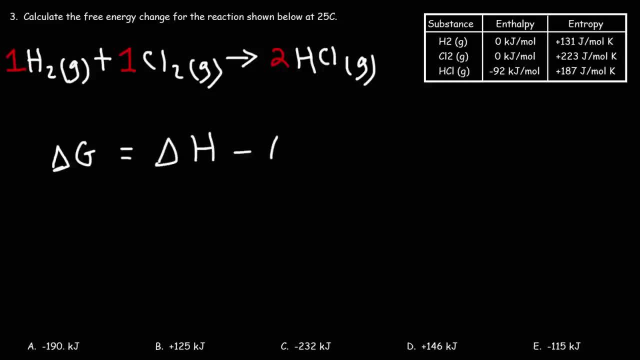 And we could use this formula: It's going to be delta H minus T times delta S. It's going to be delta H minus T times delta S. It's going to be delta H minus T times delta S. Now, using the information in this table, 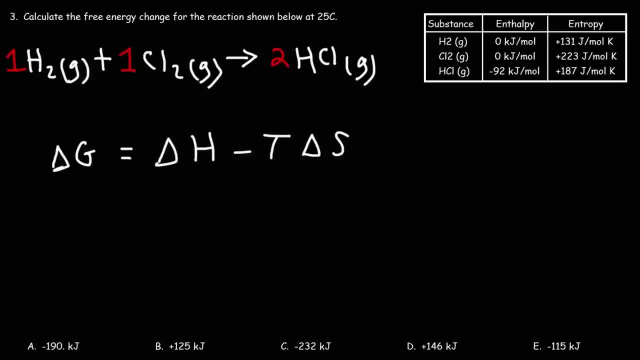 we could calculate delta H for the reaction and delta S, And once we have that we can plug it into this formula to get delta G. So let's go ahead and do that. Let's calculate the enthalpy change for the reaction. 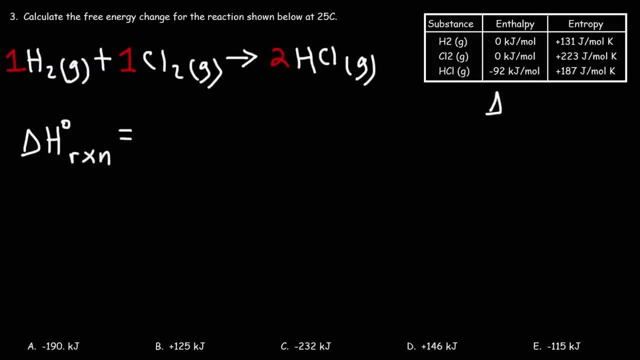 These values that you see here, they represent the enthalpy change, the energy change of formation for each of those subsets, And those values will always be zero for a pure element in its standard state. Now, the formula that we're going to use is this formula: 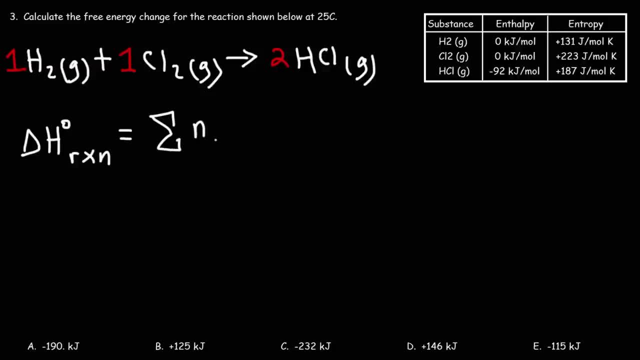 We're going to take the sum of the moles times the heat of formation for each reactor and product. But first this is going to be: this is going to be the sum of the moles times the heat of formation for each reactor and product. 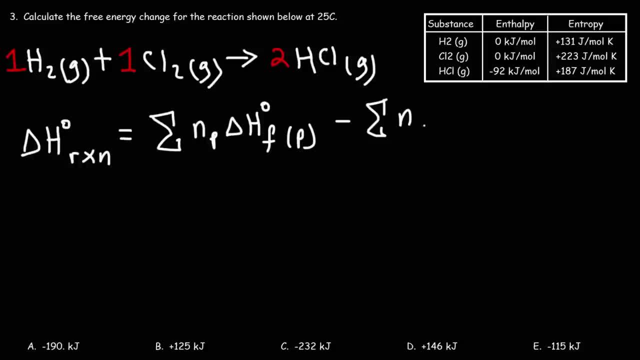 And then minus the sum of the moles times the heat of formation of all the reactants. So that's the formula we need to use. So let's start with the products. All we have is a 2 in front of HCl. 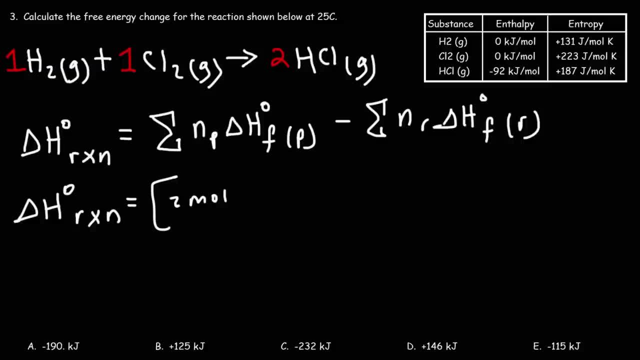 So it's going to be 2 moles of HCl. Times the heat of formation for HCl, which is negative, 92 kilojoules per mole, And then for the reactants, So for H2, we have 1 mole of that. 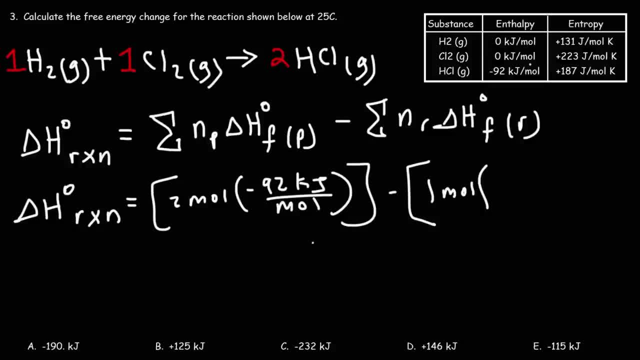 The enthalpy change for H2 is zero. For Cl2, it's 1 mole. That's the coefficient, And then times zero as well, 2 times negative 92. That's going to be negative 184. And the unit moles will cancel. 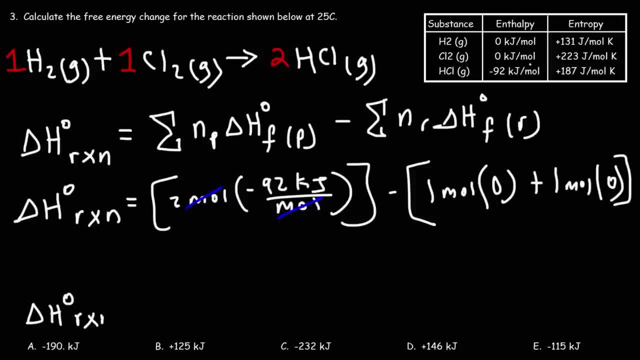 So what we have here is the delta H for the reaction. It's going to be negative 184 kilojoules, So we'll save that answer. And now let's calculate the entropy change for the reaction. So we want to get delta S at this point. 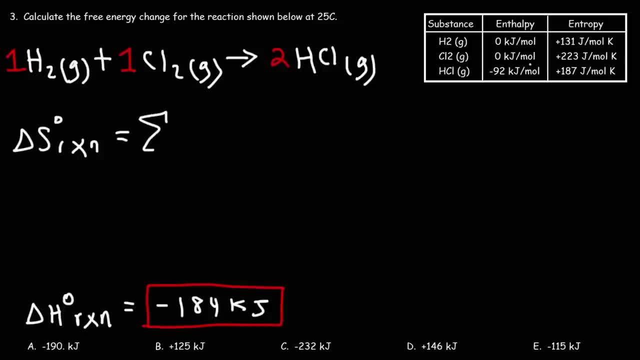 And we're going to use a similar process. So we're going to take the sum of the product of the moles times the entropy values for each product, And then we're going to take the sum of the moles of the reactants times the entropy of each product. 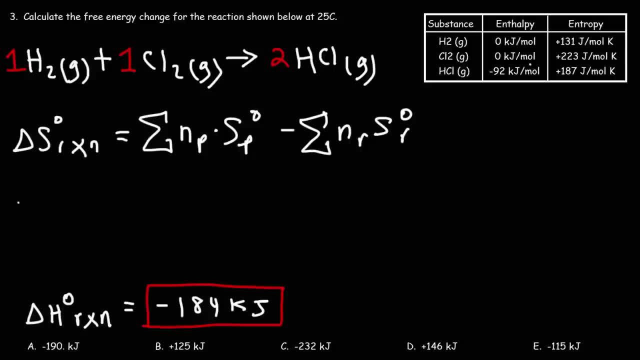 And then we're going to take the sum of the moles of each reactant. So we're going to have 2 moles of HDL And the entropy for HDL is 187.. The units being joules per mole per Kelvin. 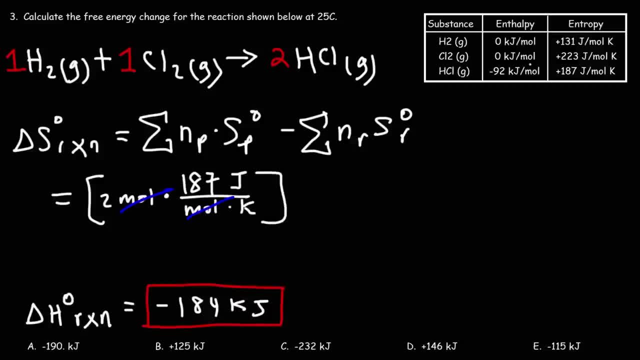 So once again, the unit moles will cancel, which will give us the entropy change in joules, Joules per Kelvin. Now let's focus on the reactants. So we have 1 mole of H2. And the entropy value for that is 131.. 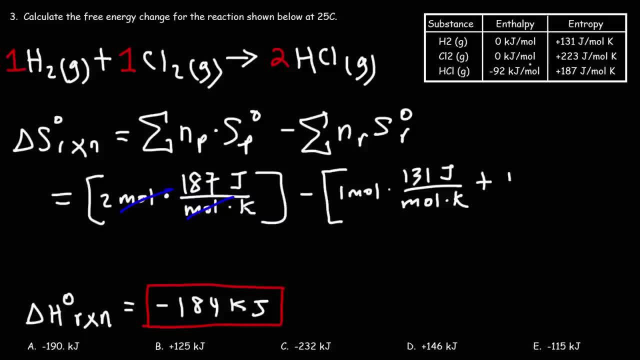 And then 1 mole of Cl2 times the entropy value for that, which is 223 joules Per mole per Kelvin. So in all cases the unit moles will cancel. So this is going to be 2 times 187 minus 131, minus 223. 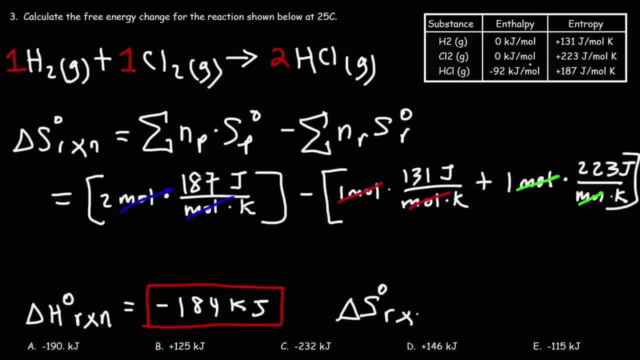 Thus the entropy change for the reaction is going to be positive 20 joules per Kelvin. Okay, So you can see that our MOL of HDL is going to be positive 20 joules. Now let's go ahead and calculate Delta G. 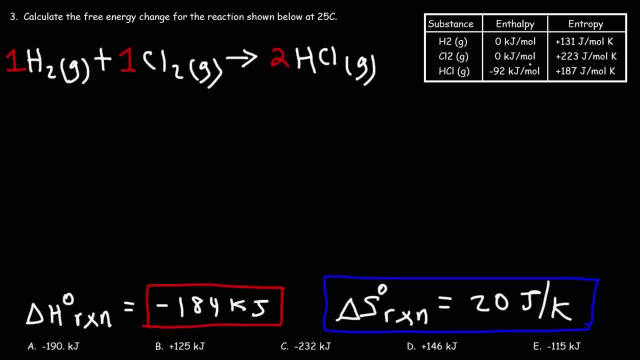 Since we now have everything that we need. So the one thing we need is the likability throughout, for the liquid, Delta G is going to be equal to swimming 3 Pray Delta H minus T times the delta S. So Delta H in this example is negative 184 kilojoules. 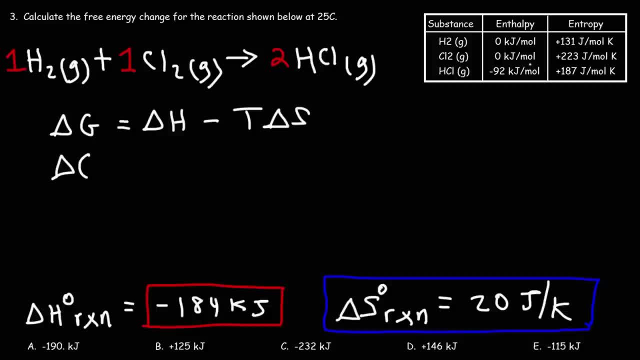 So all send determinants, and the mean of T minus TH And also delta S is going to be Tz 2 times 3 servir. Delta S being a dependentavan has its softeners should be 1.. 2. And that means that allланbene, being this vernacular German form of H2 and H3, is母소리. 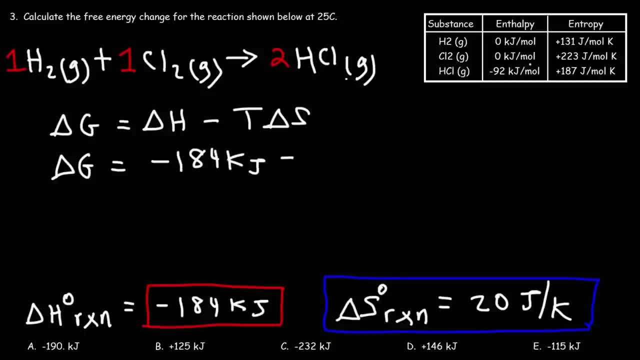 Because thelémerin or the Adénine increase the rate to tys of joules per Kelvin terms and the temperature is 25 degrees celsius, and if we add 273 to that that's going to be 298 kelvin. and then we're going to multiply that by the entropy change of not joules but kilojoules. 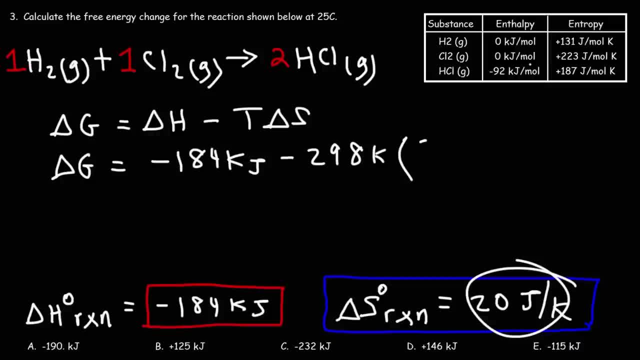 so we need to convert 20 joules into kilojoules. if we divide that by a thousand, that's going to be positive 0.02 kilojoules per kelvin. so the unit kelvin will cancel and we'll get delta g for the reaction. 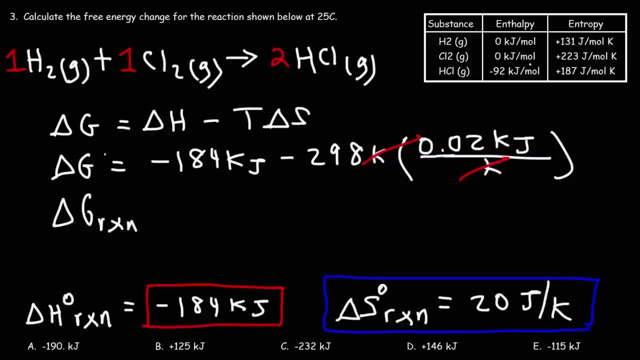 in kilojoules and this is going to be standard delta g, because we use standard delta h and standard delta s. so it's negative 184 minus 298 times 0.02. so this is going to be negative 189.92 kilojoules. so we could say that is approximately negative 190 kilojoules. 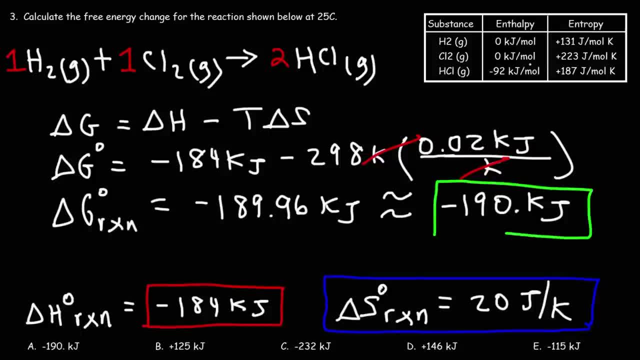 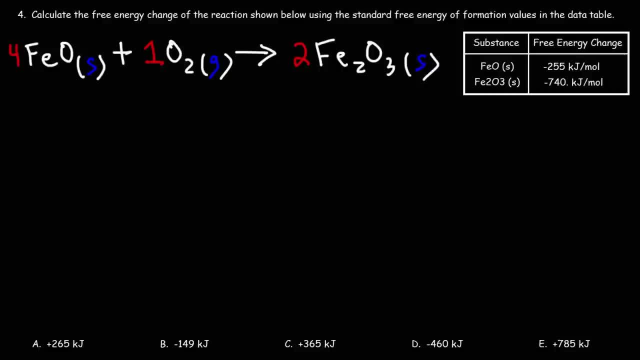 therefore, answer choice a is the correct answer. in this example number four: calculate the free energy change of the reaction shown below using the standard free energy change affirmation values in the data table. so this is going to be similar to the last problem, but we can calculate delta g directly using the table rather than the formula. 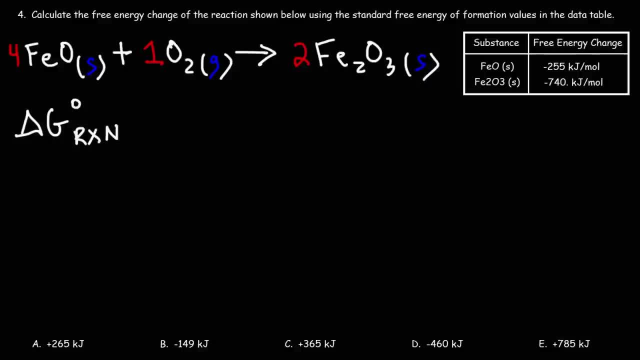 like we did in the last problem. so the free energy change for the reaction is going to be the sum of the moles times the delta g values. these are the standard delta g values of formation for all the products and then minus the sum of the moles of the reactants. 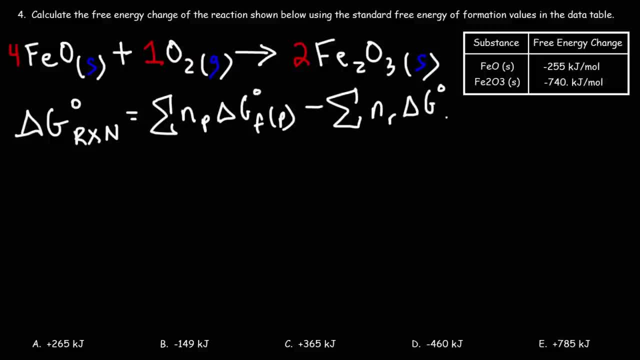 times the standard delta g values of formation for the reactants. so let's start with the products. so we have two moles of iron oxide and the value for that is negative: 740 kilojoules per mole. now for the reactants. we have four moles of rn2 oxide and we're going to 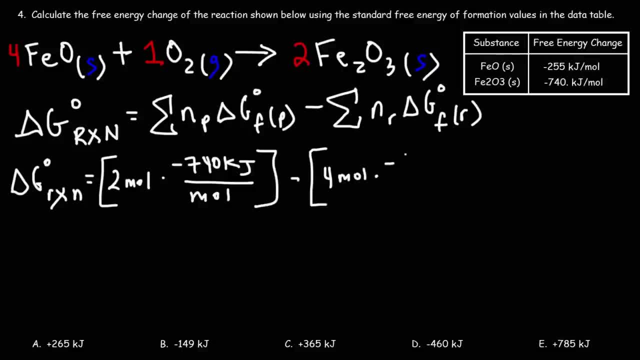 multiply that by negative 255 kilojoules per mole. now oxygen is a pure element in its standard state. so therefore the delta g of formation for that is 0.01, 0.01, 0.01, 0.01. it's going to be zero. So we could just put plus one mole times zero. So once again the 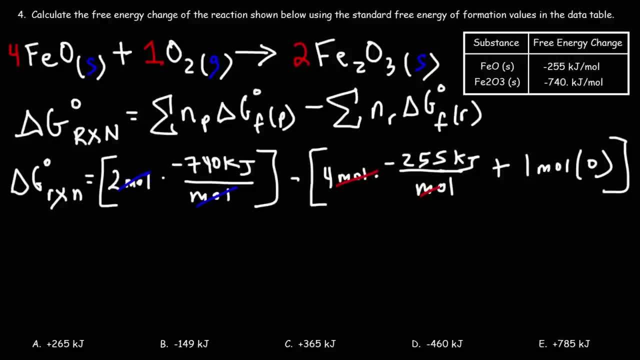 unit moles will cancel and we're going to get delta G in kilojoules. So we have two times negative: 740, minus negative 255 times 4. So I got negative 460 kilojoules. So be careful with this double negative. here There's a negative sign and another one there, So 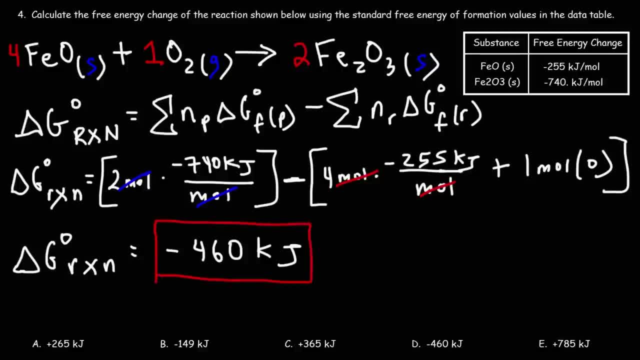 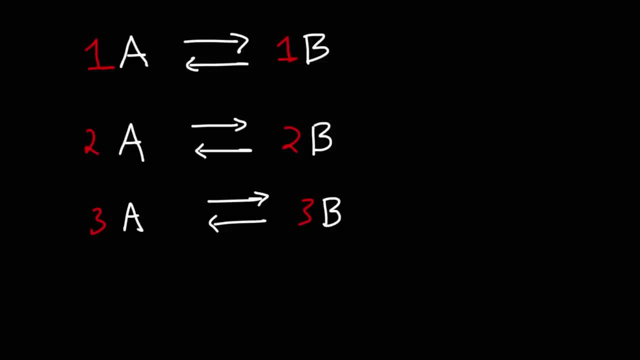 make sure you incorporate that. Thus the correct answer is going to be answer choice D. Now I want to take a minute to Mention something. When dealing with thermochemical equations, the energy change associated with a reaction, that is the amount of heat energy absorbed or released. it's typically in units. 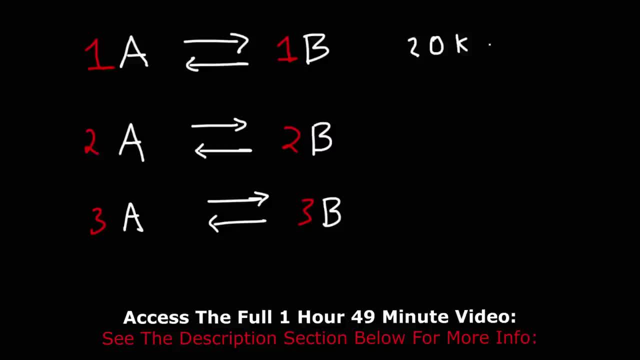 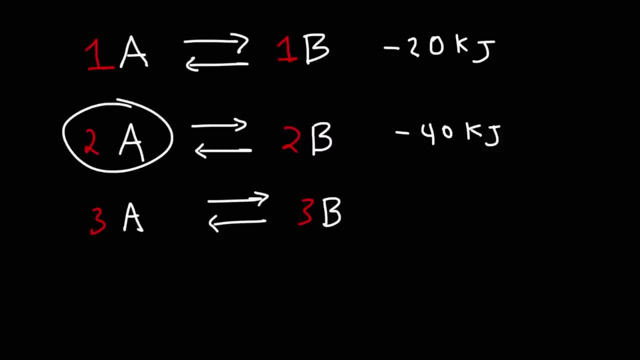 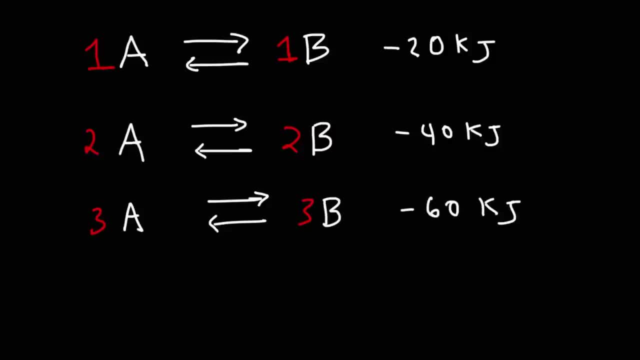 change will increase by a factor of three. Now, sometimes, instead of seeing kilojoules as the energy associated with the energy change that occurs for a reaction, you might see kilojoules per mole, And when you see that, that's basically the amount of energy that's absorbed or released. 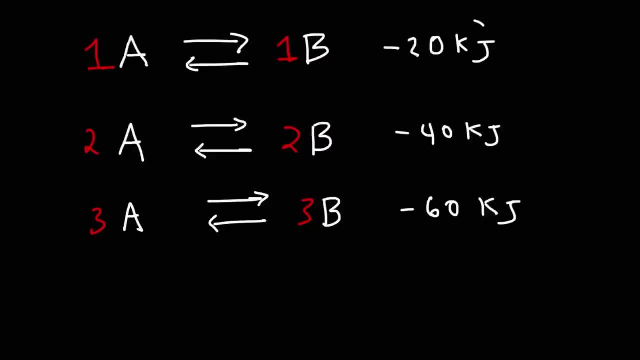 per mole of reaction. If we were to take negative 20 divided by one or one mole of A- or you can think of it as just one mole of the reaction- the energy change will be negative 20 kilojoules per mole. Now, this ratio won't change, regardless of what the coefficients of the reaction will be. 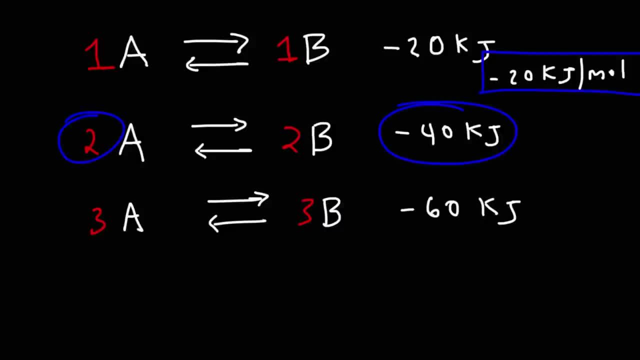 So if you take negative 40 divided by two, you're going to get negative 20. still, If you take negative 60 divided by three, you're going to get negative 20.. And when calculating the non-standard delta G value, it's important that we use this figure as opposed to these other numbers. 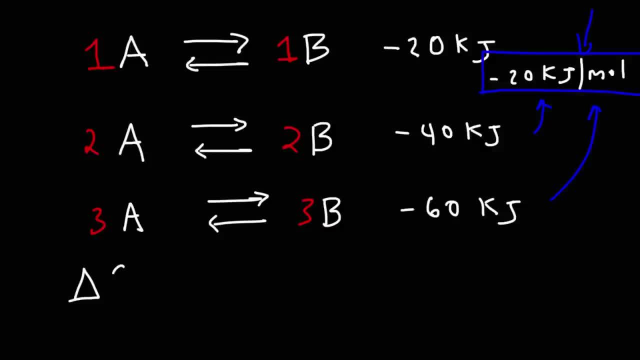 And here's why, Later in this video, we're going to use this equation. The non-standard delta G value is equal to the standard delta G value. So we're going to use this equation: The non-standard delta G value plus RT, ln, Q, where Q is the reaction quotient, R has the units joules per. 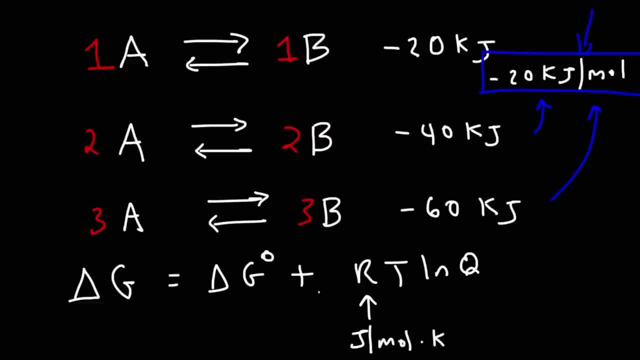 mole per Kelvin, Delta G. we can have that in kilojoules per mole or joules per mole. Temperature is in Kelvin. So in order for this equation to work, in order for us to algebraically add these quantities, they need to be in the same units. So if we were to 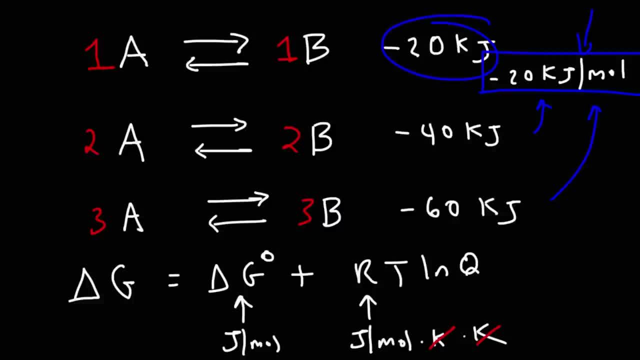 report: delta G naught as being in kilojoules and not kilojoules per mole. it won't work well with this equation, So we need it to be in joules per mole and not just joules. We can convert kilojoules. 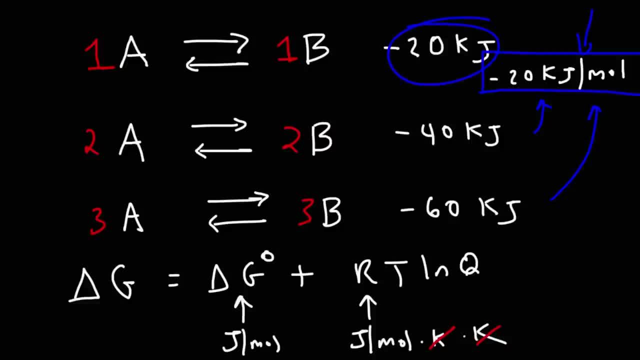 per mole to joules per mole. But if we just have kilojoules and convert it to joules, we can't add these two quantities because we need them to be in joules per mole. So going forward instead of just leaving the answer in kilojoules, let's say, if I'm calculating. 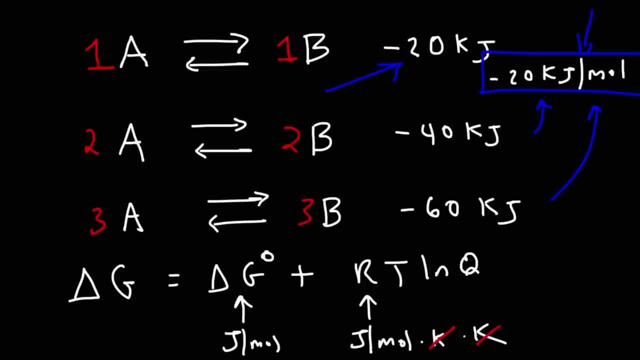 delta H or delta G of the reaction. I'm going to be using kilojoules per mole so that it works well with this equation. So I want you to be aware of those units and their relationship to each other. But for this equation to work, just make sure that delta G, naught, is in joules per mole. 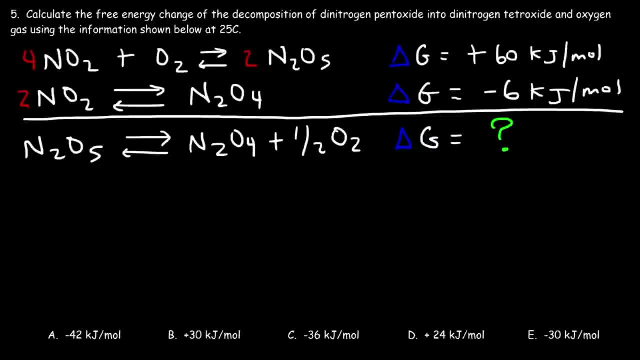 and not just joules or kilojoules. Number five calculate the free energy change of the decomposition of dinitrogen pentoxide into dinitrogen tetroxide, which is N2O4 and oxygen. So how can we use the first two equations? 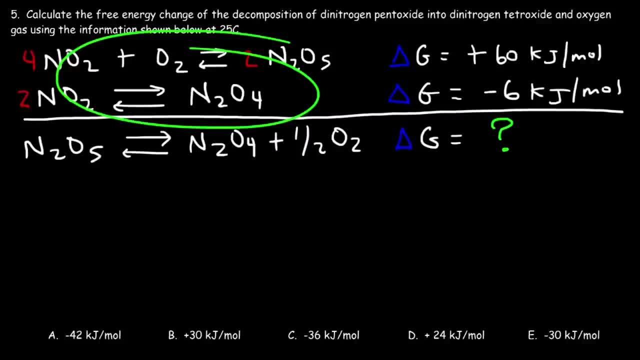 and the free energy associated with those equations to get the free energy of the third equation. What do we need to do? Well, we need to change these two equations in such a way that, when we add them, we get this equation, And so we can add the adjusted. 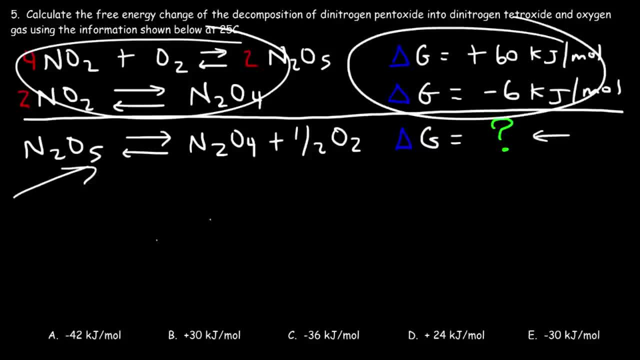 free energy change values to get this one. So how do we need to change equation one and two so that it can be added to this equation? Well, the first thing we need to realize is that notice that in the second equation, N2O4 is in the right spot and we have the right 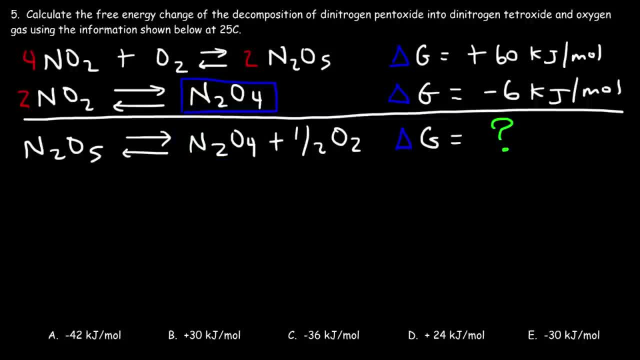 number of it. So we don't need to change the second equation Now, the first equation we do need to change: Notice that N2O5 is found on the right side, but we need it on the left And we need the coefficient to be one. So therefore the first. 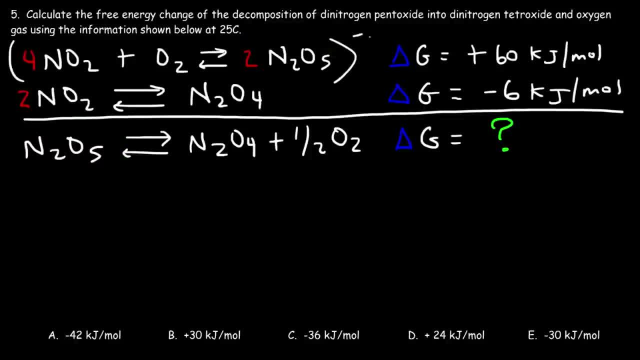 reaction. we need to reverse it and we need to multiply by half. So half of 4NO2 is going to be 2NO2.. And then we'll first need to reverse it. So let me do that first. So half of this. 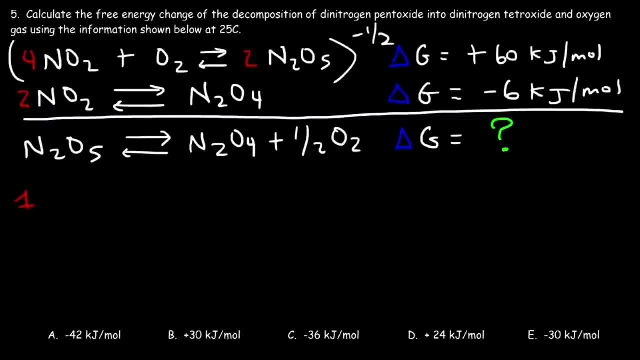 will be one, So that's 1N2O5.. And then, on the other side, half of 4NO2, that's going to be 2NO2.. And then half of O2, we can simply write that as one half O2.. Now, because we reversed it, 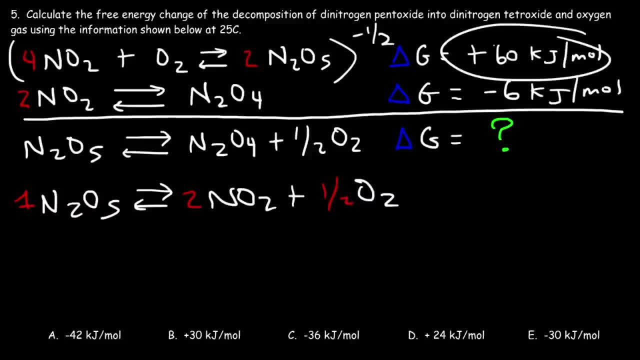 it's going to change from positive 60 to negative 60. And we multiplied it by half, Half of negative 60 is negative 30. So that's the new free energy change for this reaction. Now, this one we're not going to change, So I'm just going to rewrite it the way it is. 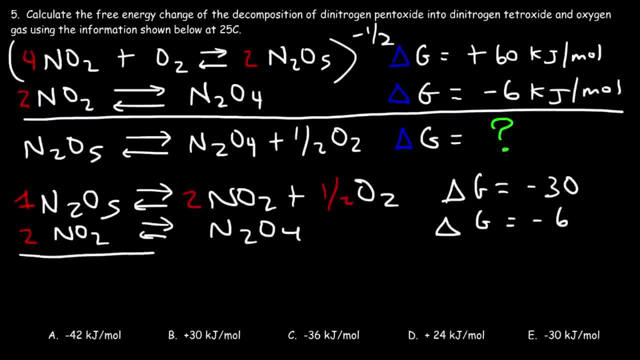 And so that's going to stay negative 6.. So now let's add these two reactions. So notice that NO2 will cancel. It's the intermediate in this reaction, And so we're left with just 1N2O5.. It turns into 1N2O4 molecule and half of an O2 molecule. So now all we need to do is add. 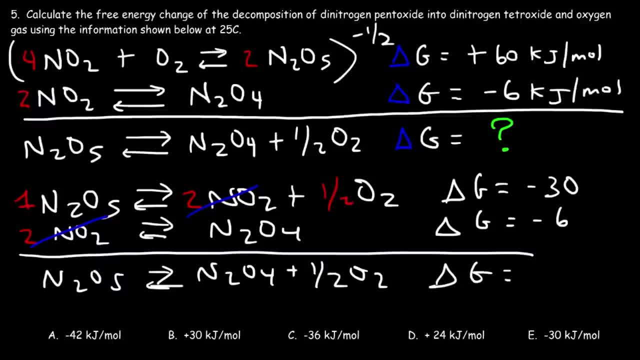 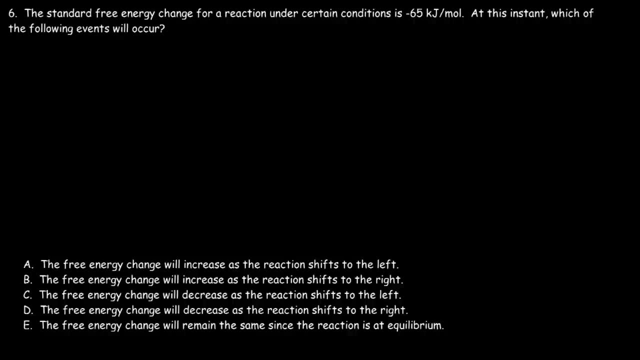 up these two values, Negative 30 plus negative 6, is negative 36 kilojoules per mole. So therefore this is the final answer. So answer choice C is the correct answer in this example Number 6.. The standard free energy change for a reaction under certain conditions is negative 65 kilojoules. 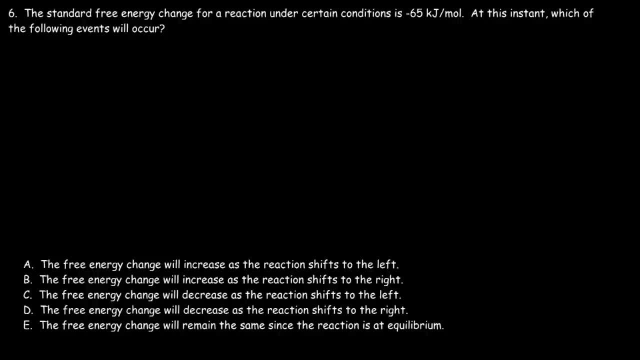 per mole At this instant, which of the following events will occur So? will the free energy change increase or decrease, and will the reaction shift to the left or to the right, or is the system at equilibrium? So let's say, if we have two species, A and B, 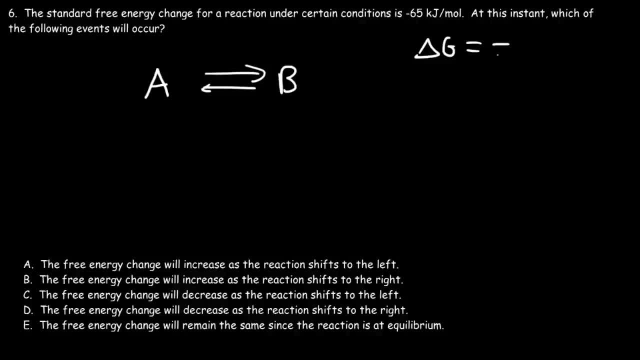 Now, if delta G is negative, what's going to happen? Is the reaction spontaneous or non-spontaneous? Anytime delta G is negative or less than zero, the reaction is spontaneous. So if we have a spontaneous process, what does that mean? 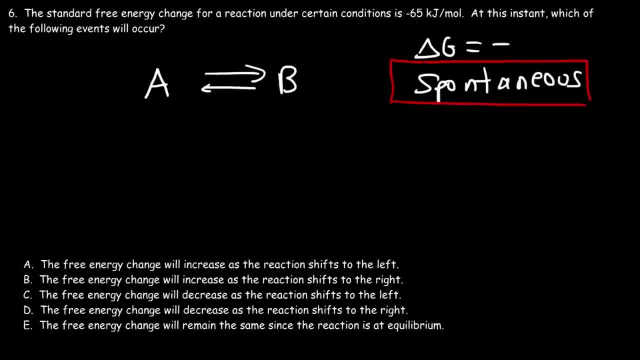 What's happening in terms of the reaction. Is the reaction going towards the right or is it going towards the left? When delta G is negative, you need to know that it's spontaneous in the forward direction. So that means that when delta G is negative, the reaction is going towards the right. 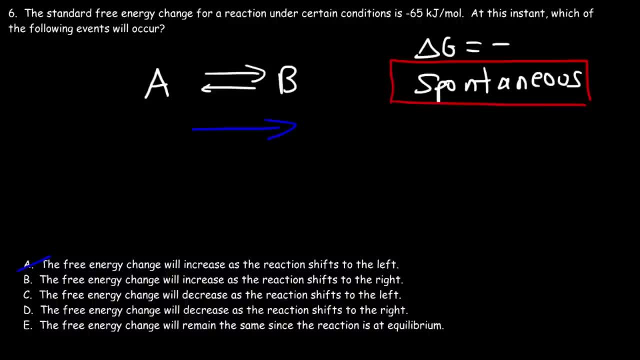 It's shifting to the right, So it's not going to the left. So A is out and C is out and it's not at equilibrium. Delta G will be at equilibrium when delta G is zero. I mean the reaction will be at equilibrium when delta G is zero. 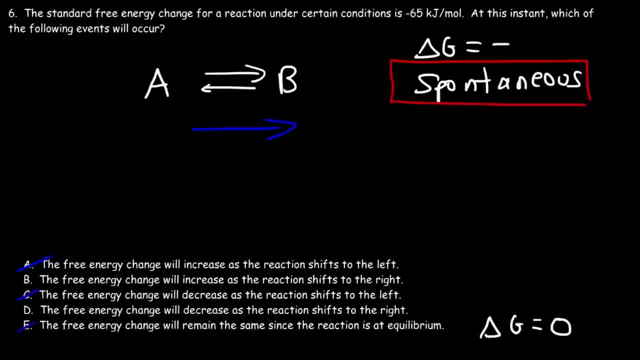 That's what I meant to say. So we're between B and D. Now, Okay, Okay, right. Will the free energy change increase or decrease? Right now, at this instant, the free energy change is negative: 65 kilojoules per mole. As the 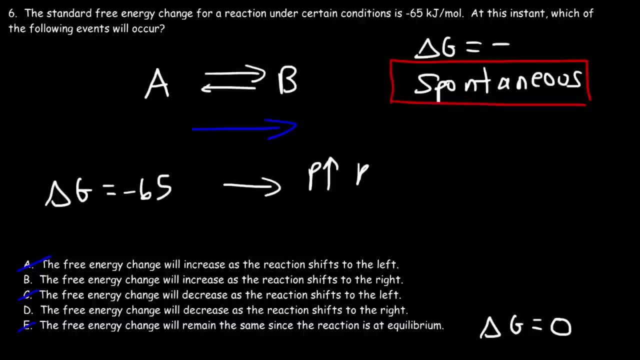 reaction shifts towards the right, the products will increase and the reactants will decrease, And this will continue to happen until it reaches equilibrium, And at equilibrium the free energy change will be 0.. So the reaction will proceed in such a way until delta G becomes 0, until the system reaches equilibrium. So 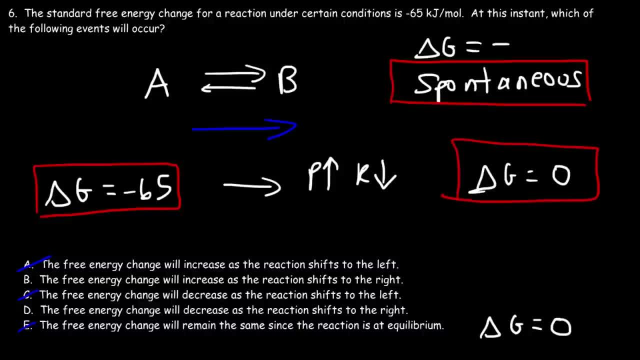 to go from negative 65 to 0,. will the free energy change increase or decrease? Well, negative 65 is a lower number on the number line relative to 0. So let's say, if you draw a number line, Here's 0,, here's 50,. 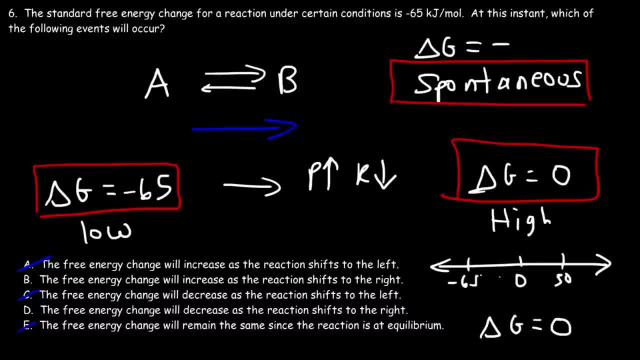 here's negative 65. The lower numbers on the left side. So therefore delta G has to increase from negative 65 to 0 as the reaction proceeds to the right, going towards equilibrium. So therefore we can eliminate answer choice D. It's not going. 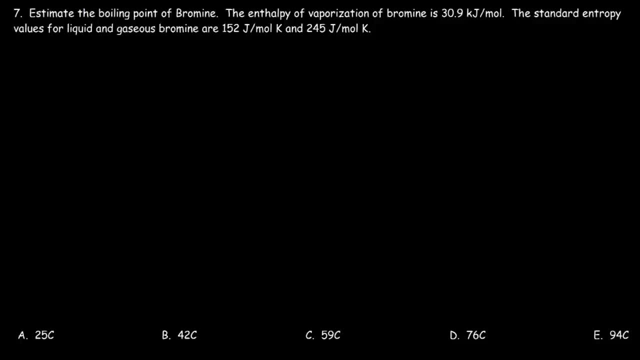 to decrease, it's going to increase. Number seven estimate the boiling point of bromine. Now we're given the enthalpy of vaporization of bromine- it's 30.9 kilojoules per mole- and the standard entropy values for liquid and gaseous. 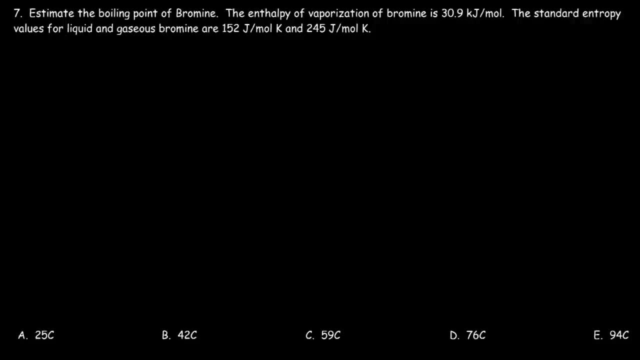 bromine are 152 and 245 joules per mole per Kelvin. Now let's write a reaction. So we have liquid bromine turning into gaseous bromine, And so the enthalpy of vaporization is basically the enthalpy of this reaction, because liquid bromine 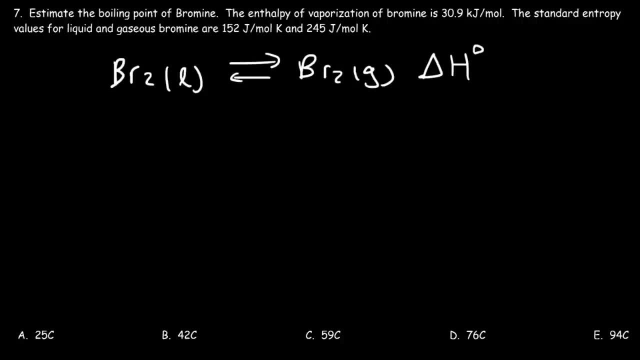 is being vaporized into gaseous bromine. So the entropy of vaporization is basically the entropy of this reaction, because liquid bromine is being vaporized into gaseous bromine, So the enthalpy of the reaction is positive: 30.9 kilojoules per mole. Now how can we? 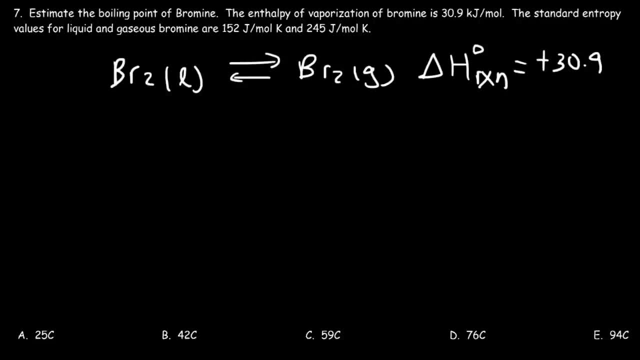 calculate the boiling point of bromine. What do we need? Well, we need to start with this equation: delta G is equal to delta H minus T, delta S, And at the boiling point, these two physical states coexist. So what that means is that this: 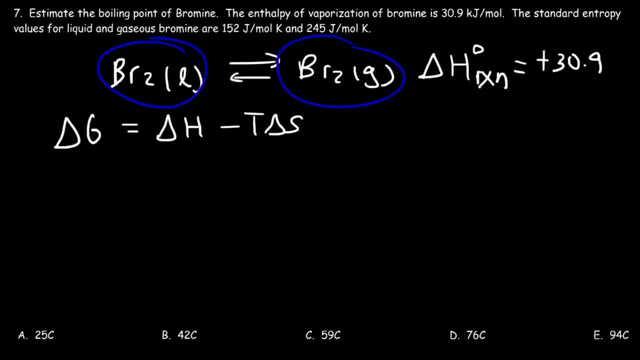 system is an equilibrium. at the boiling point The liquid state and the gaseous state, they coexist. They can go back and forward at that temperature. Now, if this system is an equilibrium, what is delta G? At equilibrium, delta G is equal to zero. So now what we have is zero is equal to. 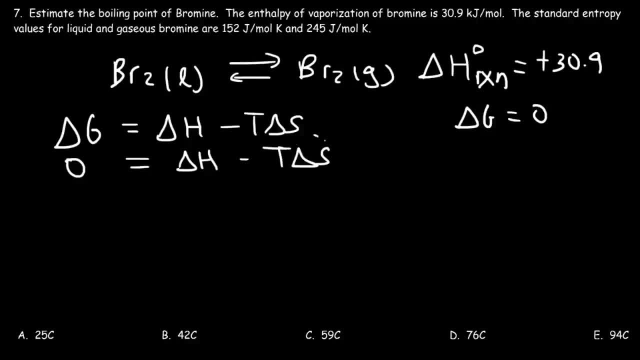 delta H minus T Delta S. So let's take this term and move it to the other side. So T Delta S S is equal to delta H, And now we need to calculate T, And T represents the boiling point temperature, And so to calculate it, it's simply the enthalpy of vaporization divided. 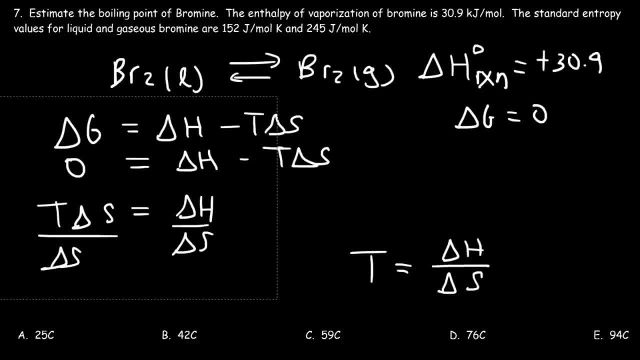 by the entropy change. So that's how you can calculate the boiling point of a liquid. Now we already have the enthalpy change. What we're missing is the entropy change. So to calculate the entropy change for the reaction, it's going to be the sum of the entropy values. 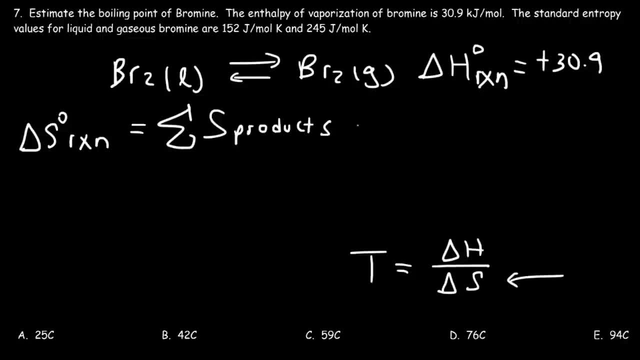 for the products minus the sum of the entropy values for the reactants. Now, the only product that we have in this reaction is gaseous bromine, So I'm going to write G for gas And the reactant is liquid bromine, And the entropy value for gaseous. 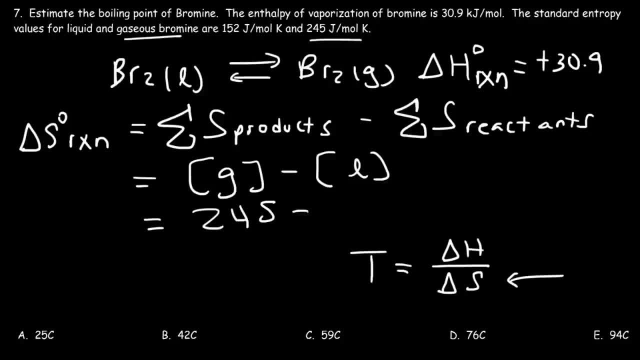 bromine is 245.. And for liquid bromine it's 152.. So let's subtract those values, 245 minus 152. And so the entropy change is 93. And the units are joules per mole per Kelvin. So now we have the entropy change And we 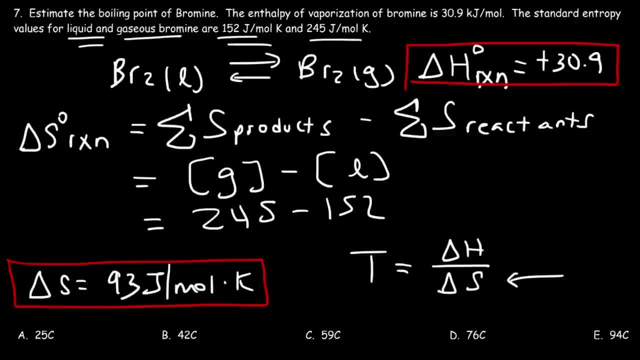 have the enthalpy change. So with that information we can go ahead and calculate the temperature. Now we need to be careful with the units. As you can see, the entropy change is in kilojoules per mole. The entropy change is in joules per mole, So I'm going to convert this to: 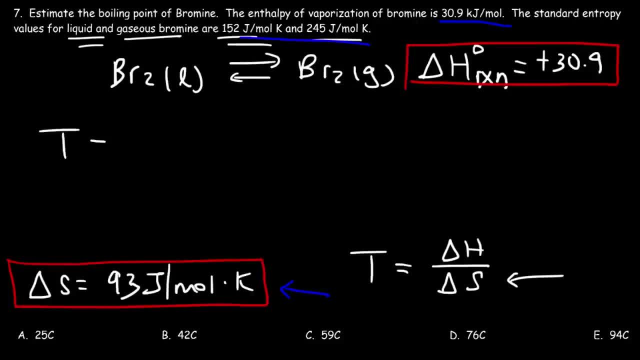 kilojoules by dividing it by 1,000.. So the temperature is going to be the entropy of vaporization, which is 30.9 kilojoules per mole divided by the entropy change, 93 divided by 1,000. That's 0.093.. And it's going. 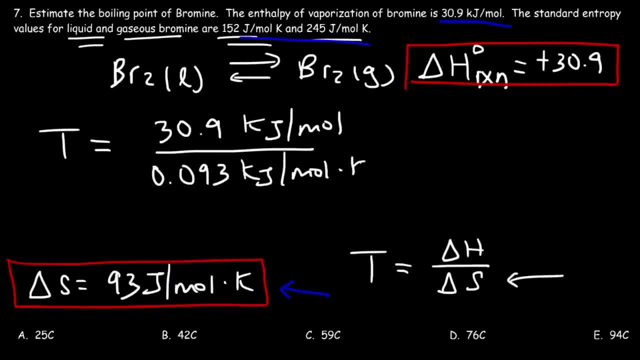 to be kilojoules per mole per Kelvin. So we can see that the unit kilojoules will cancel and the unit moles will cancel, And so we're going to get the temperature in Kelvin. So it's going to be triple nine divided by 0.093.. Now this is equal to 332.26 Kelvin. And if 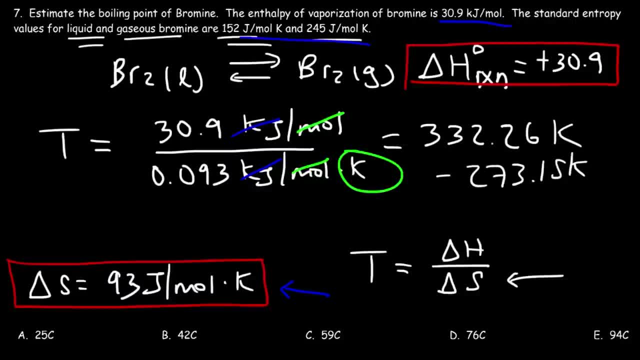 we subtract this by 273.15 Kelvin, we can convert it to Celsius. So the temperature is about 59.1 degrees Celsius. So we can route it and say the boiling point of bromine is approximately 59 degrees Celsius. therefore, C is the right answer in this. 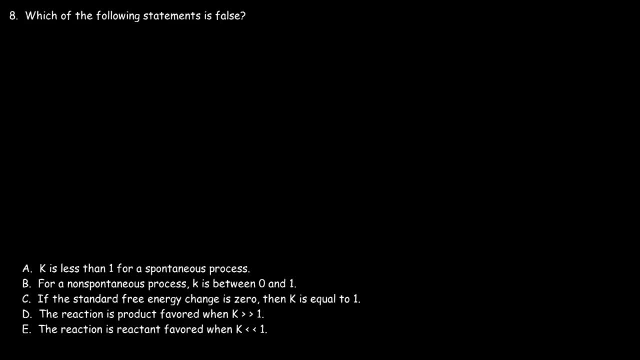 problem number 8: which of the following statements is false? is it a, B, C, D or E? well, let's go over some things that you need to know now. when Delta G is less than zero, that means it's negative. we have a spontaneous reaction, and so that. 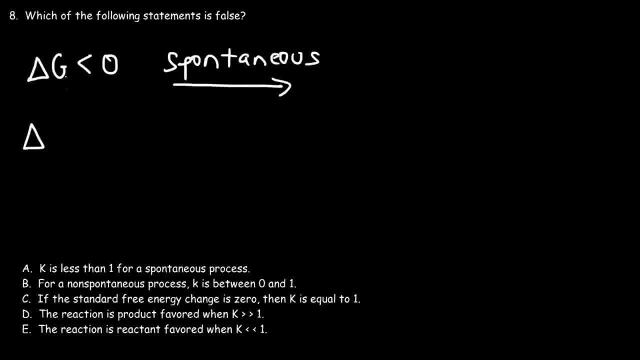 means that the reaction shifts to the right. if the standard Delta G value is equal to zero, then that means that the system is at equilibrium, and if the standard free energy change is greater than zero, then we have a non spontaneous reaction. it's non spontaneous in the forward direction, which means it's 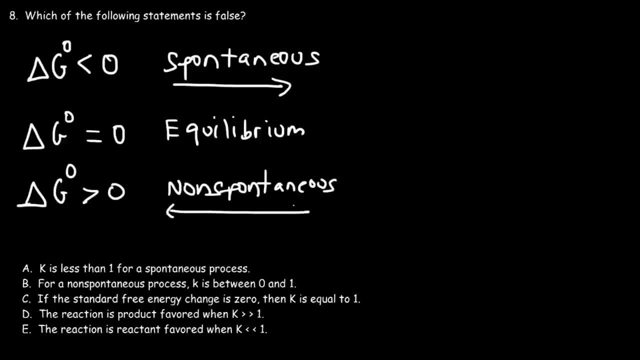 spontaneous in a reverse direction, so it shifts the left. Now keep in mind: when delta G is less than 0, it's equivalent to being negative, And when delta G is greater than 0, it's equivalent to being positive. Now, when we have a spontaneous reaction, when delta G is less than 0, then K is. 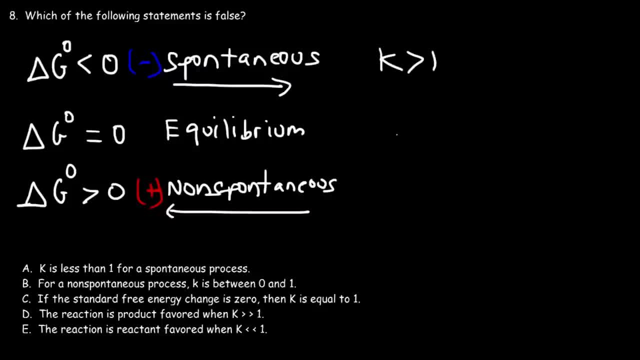 greater than 1.. And at equilibrium, K is equal to 1.. And if we have a non- spontaneous reaction, K is less than 1, but it has to be greater than 0.. K cannot be a negative number. Now, when K is greater than 1, it's product favored, Keep in mind. 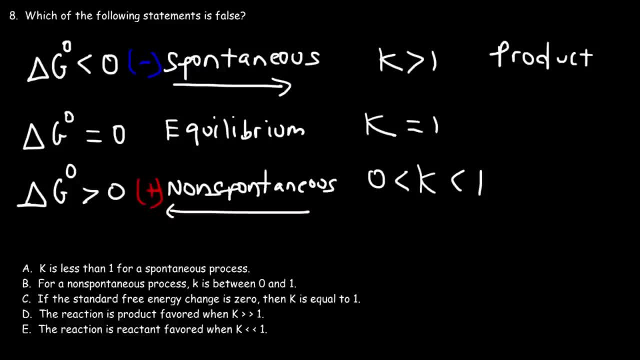 K is the ratio of the products to the reactants. So let's say, if K is a significantly large number, like 10,000. That means that at equilibrium there's a lot more products than reactants. So anytime the reaction shifts to the right, 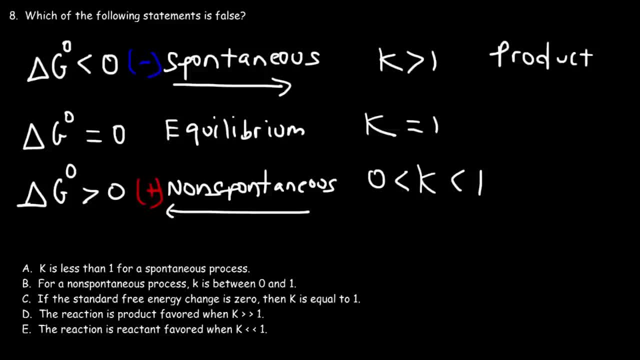 for a spontaneous process. it means that it's product favored If delta G is positive. where K is small, like 1 times 10 to negative 8 or something, you have a non-spontaneous process, So it's spontaneous in the reverse direction. So it's reactant favored when K is small. 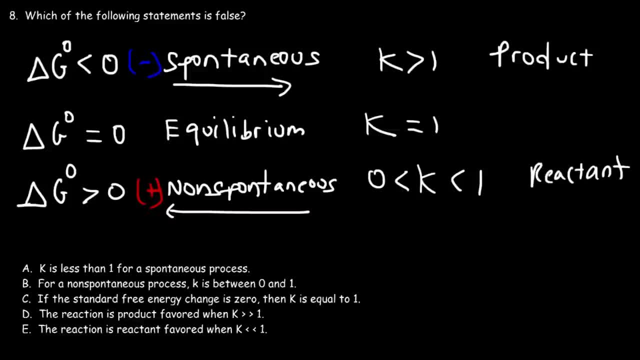 but it's product favored when K is large. So if we look at E, the reaction is reactant favored when K is significantly less than 1.. That's true. And D, it's product favored when K is significantly larger than 1.. 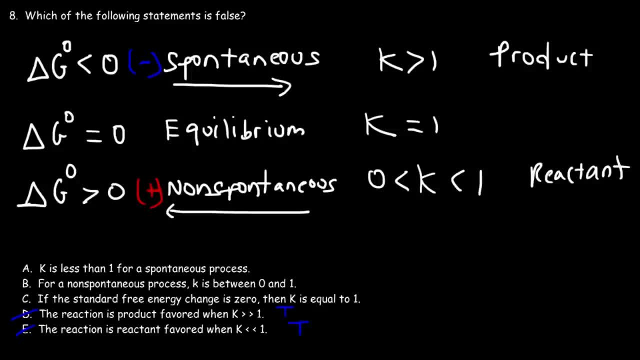 That's also true. Answer choice C: if the standard free energy change is 0,, then K is equal to 1.. That is a true statement. And for B, for a non-spontaneous process, K is between 0 and 1.. And that's just something you need to know. So make sure. 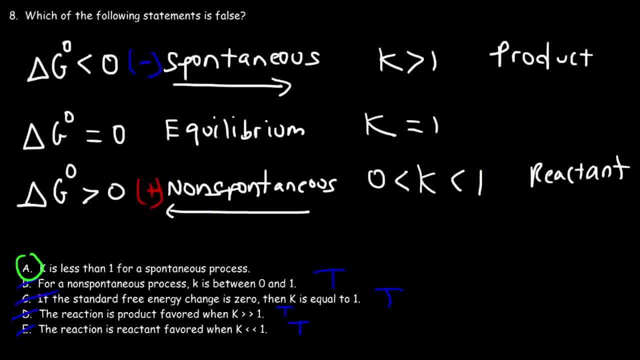 you write that down in your notes. Now A has to be the false statement. For a spontaneous process, K is not less than 1.. In fact, K is greater than 1 when spontaneous, because delta G is negative is less than 0. So A is the correct answer. is the statement that is false. 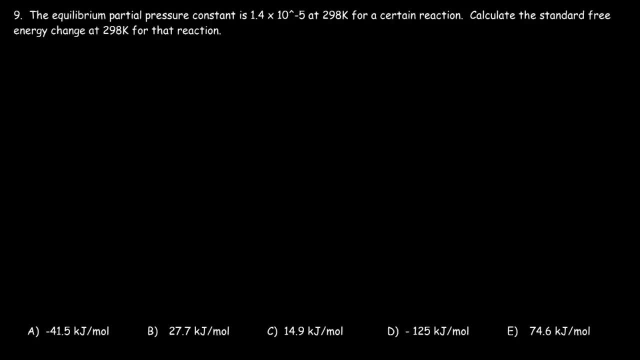 Number nine. the equilibrium partial pressure constant is 1.4 times 10 to negative 5 at 298 Kelvin for a certain reaction. Calculate the standard free energy change at 298 Kelvin for that reaction. So we're given Kp, the equilibrium partial. 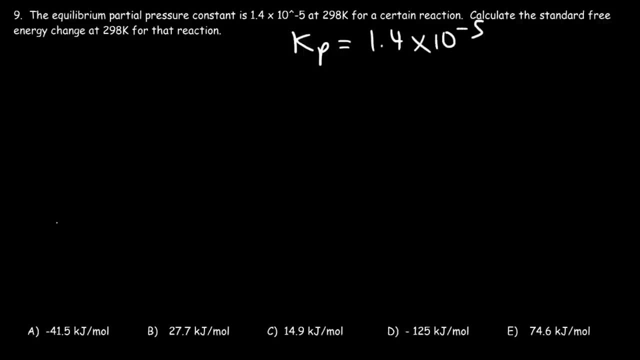 pressure constant and it's equal to this value. so how can we use this number to calculate Delta G? now there is a formula: the standard free energy change is equal to negative RT times the natural log of the equilibrium constant. so R in this example is the energy constant eight point three, one, four, five joules per 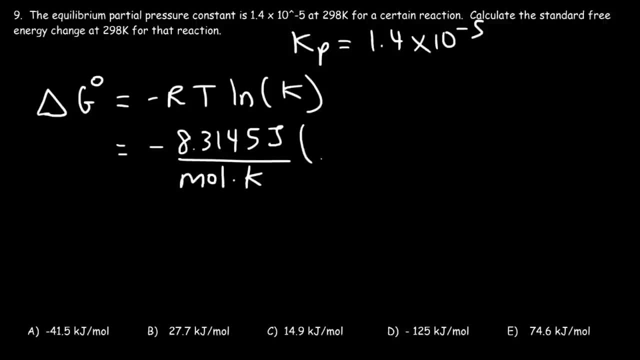 mole per Kelvin, and the temperature in Kelvin is 298 Kelvin, and so we can see that the units Kelvin will cancel and K is unit list, so we don't have to worry about that. now the units that we're going to have is joules per mole and 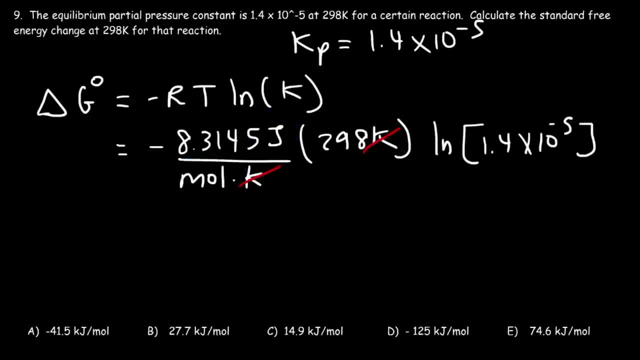 Delta G has to be in kilojoules per mole, so we need to convert it to that. so let's take a negative eight point three, one, four, five, multiply by two and that's going to give us the value of delta G, which is divided by 298 times the natural log of 1.4 times 10 to negative 5, so the 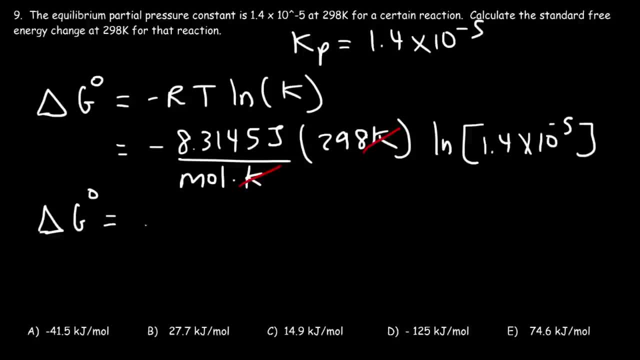 standard free energy change for this reaction is positive: 27,700 joules per mole. if you round it now, let's convert it to kilojoules per mole. so one kilojoule is 1,000 joules and now we can cancel this unit. 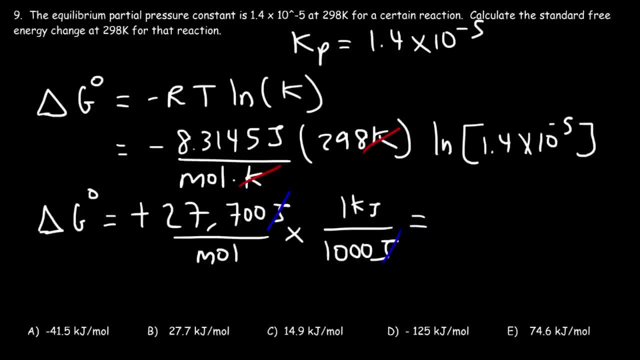 you. so 27,700 divided by a thousand is 27.7 kilojoules per mole, and so that's Delta G in this problem, which means that B is the right answer. now let's think about this. notice that K is very small. it's point zero, zero, zero zero one four, so K. 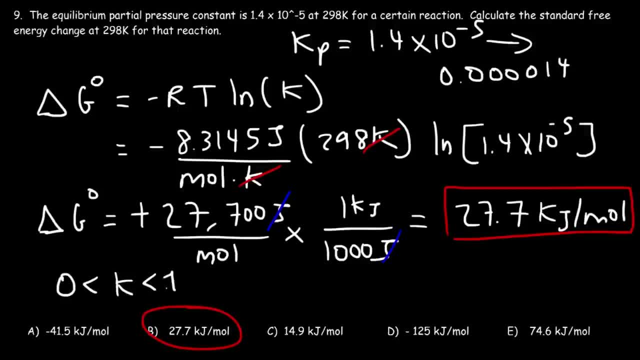 is greater than zero, but it's less than one, which means that we have a total of the reaction and notice that Delta G is positive. we said that if K is less than one, delta G is positive, or delta G is greater than zero, which means that it's. 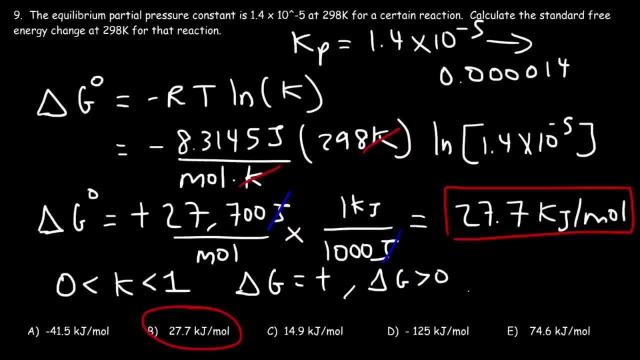 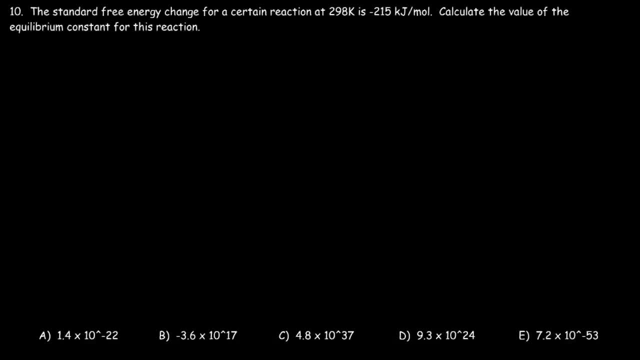 non spontaneous in the forward direction, but it is spontaneous in a reverse direction, so it's reactant favored. it goes towards the left. number 10: the standard free energy change for a certain reaction at 298 Kelvin is not negative: 215 kilojoules per mole. calculate the value of the equilibrium. 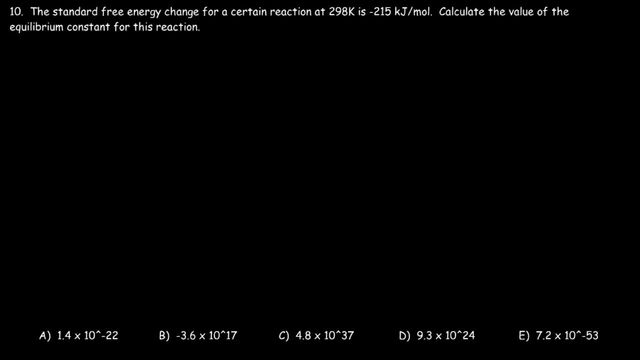 constant for this reaction. so how can we do this? what should we do now? notice that Delta G is equal to a negative number and we know that when it's negative, the reaction is spontaneous, it's going to shift to the right and it's a product favored reaction. 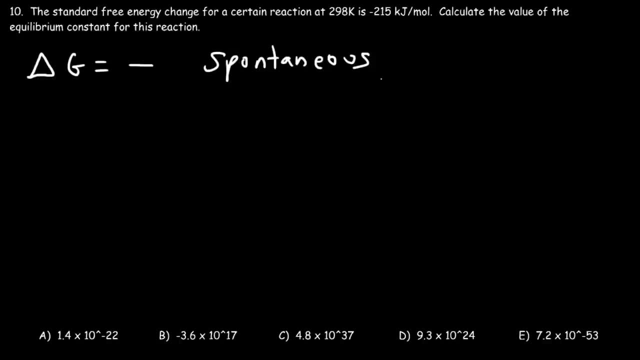 now, when Delta G is negative, is K very large, very small if its product favored, K is going to be very large. so K is going to be a positive number and it's going to be 10 raised to some positive exponent. it's a large number on the. 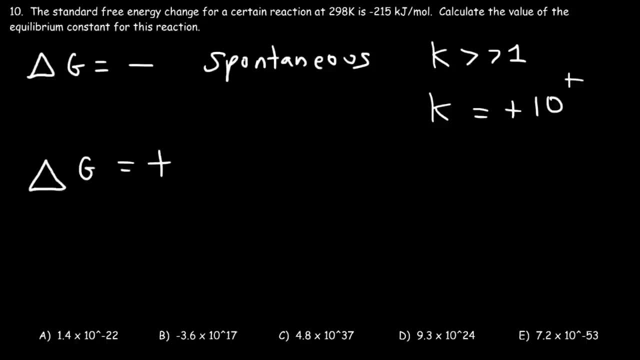 other hand, when Delta G is positive, we have a non spontaneous process, and so the reaction is reactant favored, and so K is going to be less than one, but greater than zero. so because it's greater than zero is still a positive number, but it's less than one, so the exponent has to be negative as opposed to. 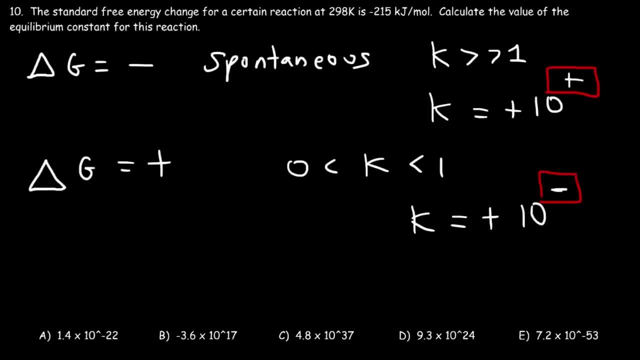 being positive, but for this problem Delta G is clearly a negative value. so we need a positive K value. with a positive exponent we can eliminate answer choice a because it has a negative exponent, which means that Delta G is positive. this also has a negative exponent. now K can never be negative, so B is out. so it's either between C or D, that's. 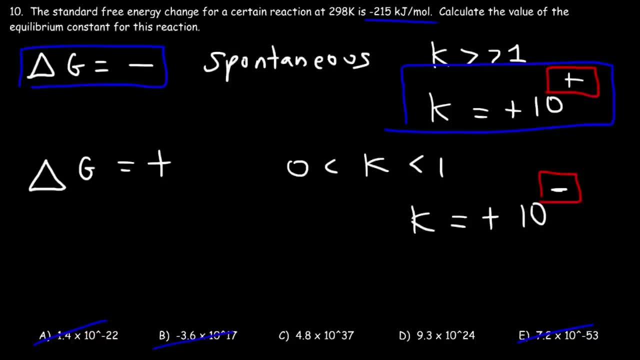 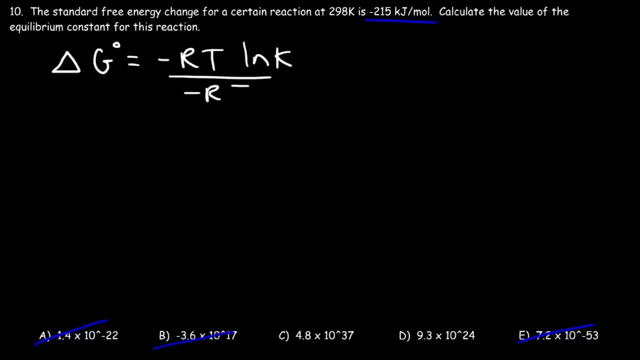 when K is positive and has a positive exponent. but let's get the exact answer now. let's start with this equation: Delta G is equal to negative RT LN K. so the first thing we need to do to isolate K is to divide both sides by a negative. 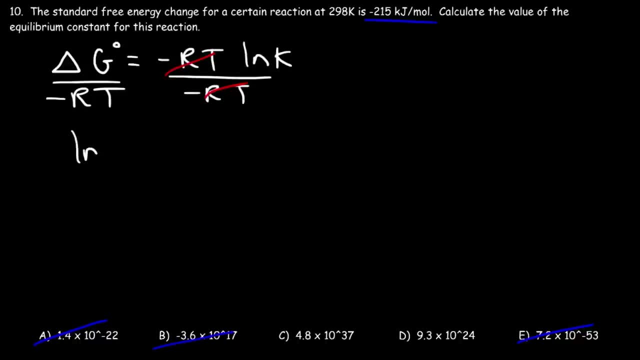 RT, And so LNK is equal to negative delta G over RT. Now we need to get K by itself. When dealing with logarithms, here's some general things you need to keep in mind. A raised to the C is equal to B, So that's how you can convert a logarithmic expression into: 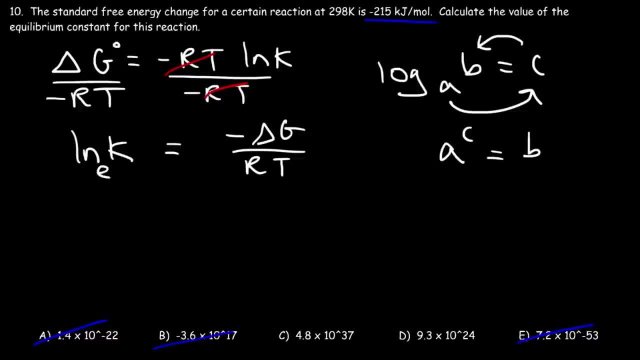 its exponential form. Now, the base of a natural log is E. So E raised to everything on the right side is equal to K. Or we could say K is equal to E raised to the negative delta G over RT. So that's the formula that we're going to use to calculate K. 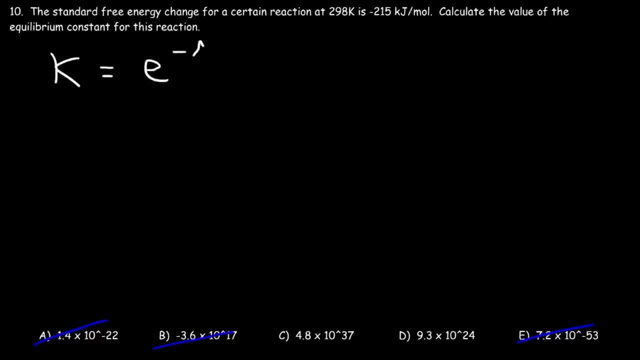 So I'm just going to rewrite it here Now: when using this formula, because R is in joules per mole, delta G has to be in joules per mole, So you got to convert kilojoules to joules, So let's do that first. So we have negative 215 kilojoules per mole. 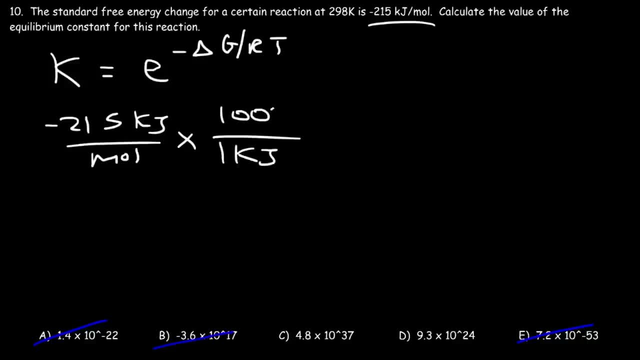 And we know that one kilojoule is equal to a thousand joules. So this time we need to multiply by a thousand as opposed to divide by a thousand. So it's negative 215,000 joules per mole. So K is going to be E negative 215,000.. Now that's delta G, And keep in mind 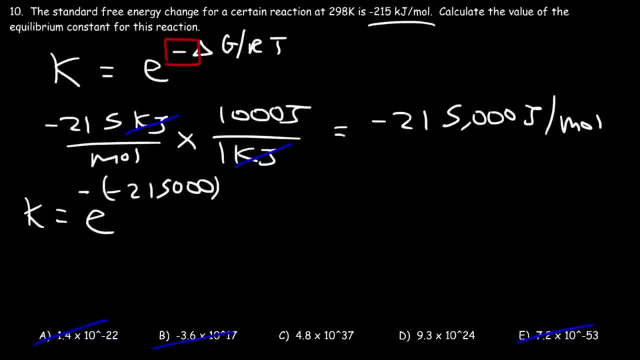 there's another negative sign, So it's negative delta G. So we got two negative signs in this example. And then R, which is 8.3145, multiplied by the Kelvin temperature, 298.. Don't plug in a Celsius temperature, You won't get the right answer. And so this is equal to 4.8 times 10. 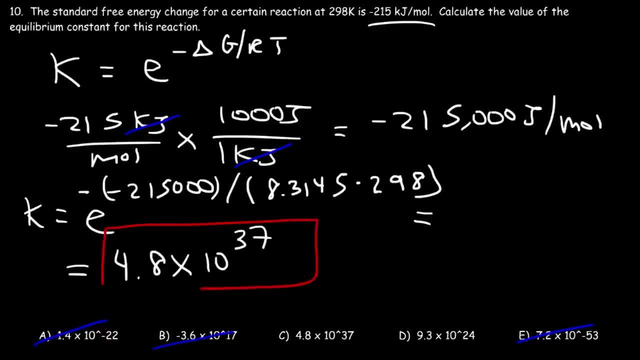 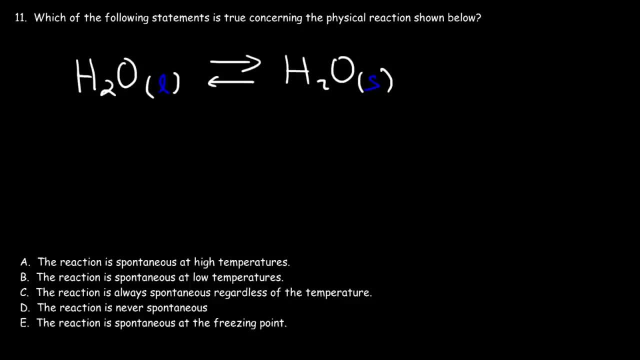 to the 37th. So that's the value of the equilibrium constant. So C is the answer for this problem, Number 11.. Which of the following statements is true concerning the physical reaction shown below? Is the reaction spontaneous at high temperatures, low temperatures? Is it always spontaneous? and 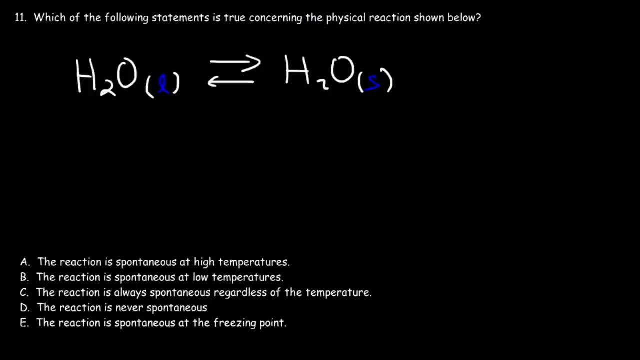 never spontaneous, Or is it spontaneous at the freezing point? So in this reaction we have a constant and we have a high temperature, And if we have a high temperature we have a liquid water turning into ice. so which statement is true? if we take a step back, 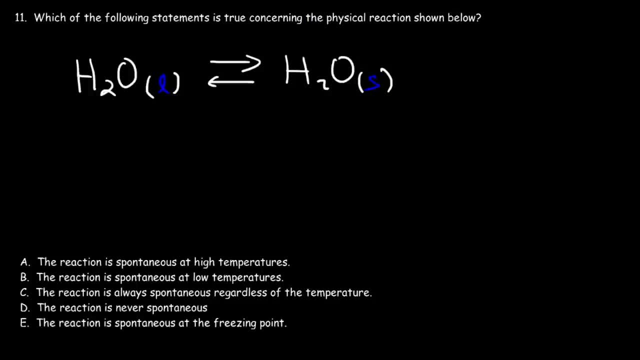 and keep it simple. the best way to turn liquid water into ice is to put it in a freezer. if you put it in a freezer, heat energy is going to flow away from the liquid water, and so, as water loses thermal energy, the temperature decreases, and as the temperature decreases, it's 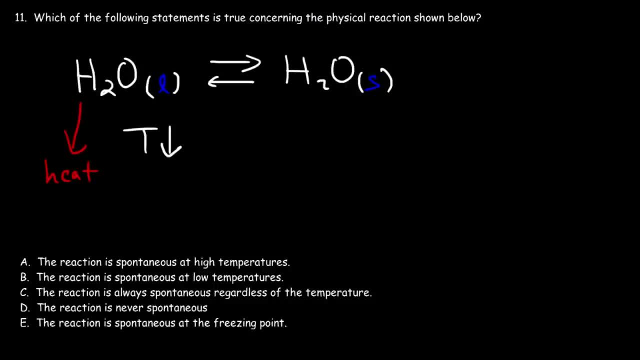 going to freeze to ice. so therefore we know that it's spontaneous at low temperatures. so just by intuition, you know that the answer has to be B. but now let's talk about why that's the case. so first, this reaction: is it endothermic or exothermic? the freezing of water in 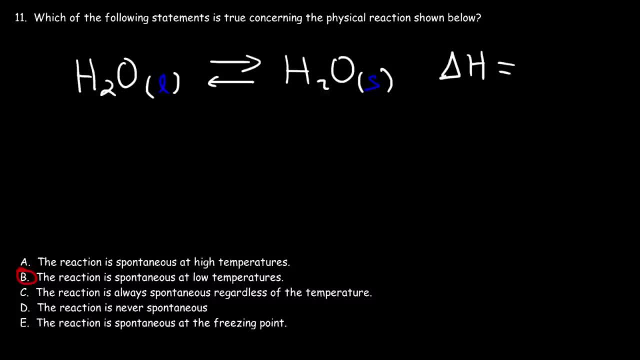 order to freeze water, in order to go from a liquid to solid, you need to remove energy, so liquid water has to release heat energy into the surroundings. so let's say we have a beaker filled with liquid water if we put it in a freezer with, let's say: 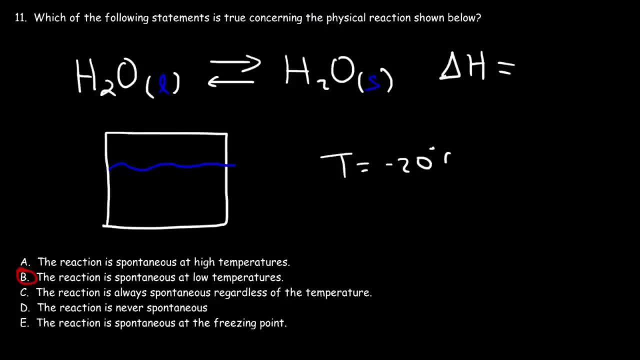 the temperature is negative 20 degrees celsius and the temperature of this water is 25. heat flows from hot to cold, so heat is going to leave the system and it's going to flow into the surroundings. when the system releases heat energy, it's an exothermic process. so Delta H is 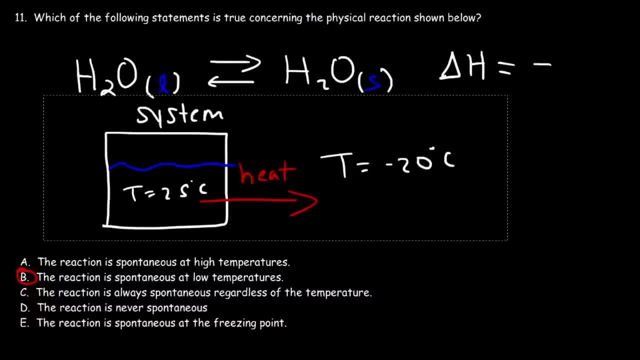 negative. now the next thing we need to analyze is the entropy change. is it positive or is it negative? so which one has more entropy, a solid or liquid? a solid is very organized. it doesn't have much disorder, so a solid has a very low entropy value. a liquid has a relatively 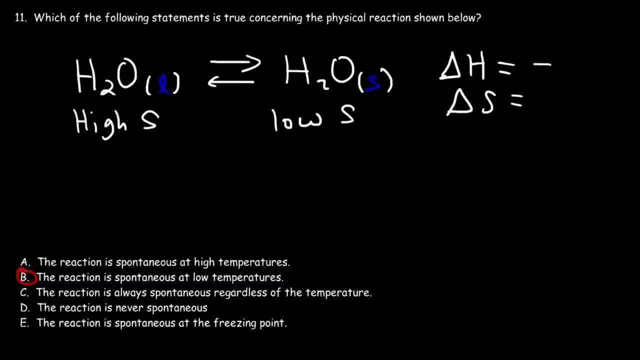 higher entropy value than the solid a, so going from a high entropy value to a low entropy value, so entropy is decreasing. therefore, Delta S is also negative. now you need to be familiar with this table: Delta H, Delta S, T and Delta G. you may want to commit this to. 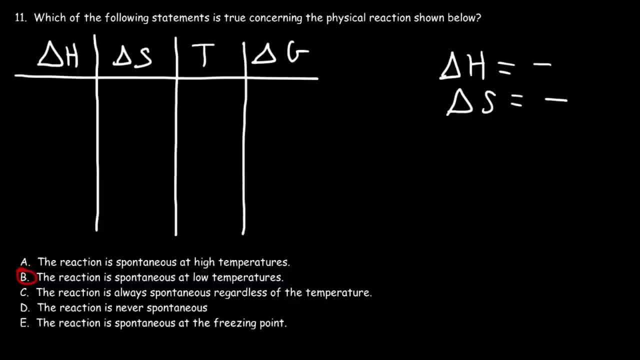 memory. so when Delta H and Delta S are both positive or both negative, the sign of Delta G is temperature dependent. so when they're both positive and the temperature is high, Delta G is going to be negative, which means that it's spontaneous. under these conditions it's. 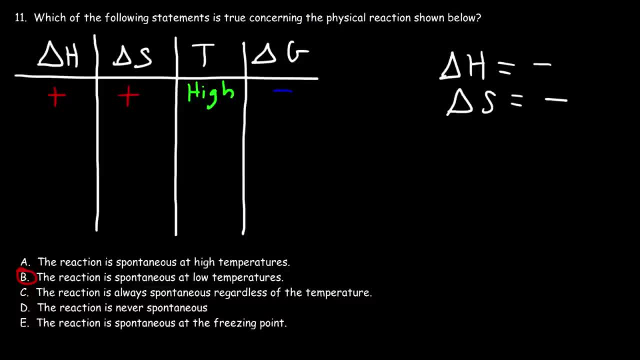 spontaneous at high temperatures and it's non-spontaneous at low temperatures. now, when Delta H and Delta S are both negative, it's still going to be temperature dependent. this time, Delta G is negative at low temperatures, so it's going to be spontaneous at a low. 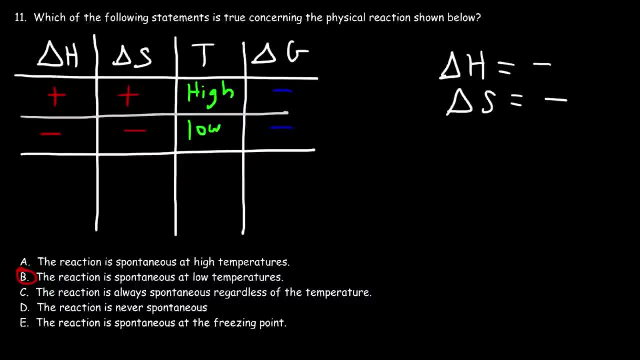 temperature, but non-spontaneous at a high temperature. now, when the signs of Delta H and Delta S are different, then it's no longer temperature dependent. so when Delta H is negative and Delta S is positive, Delta G is always positive, spontaneous, regardless of the temperature, and when Delta H is. 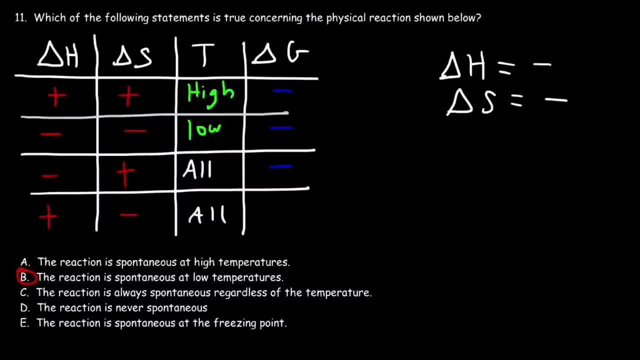 positive and Delta S is negative. it's always going to be non-spontaneous. so in this example, Delta H and Delta S are both negative, so we're dealing with this section here. so the reaction is going to be spontaneous only at low temperatures and it makes sense, liquid water will. 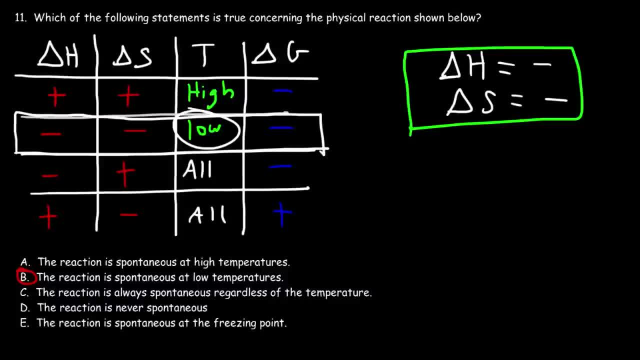 only freeze at low temperatures. so that's why B is the answer. we can eliminate A. it's not going to be spontaneous at high temperatures, and C and D doesn't apply. now what about E at the freezing point, that is, if the temperature is zero degrees Celsius? then